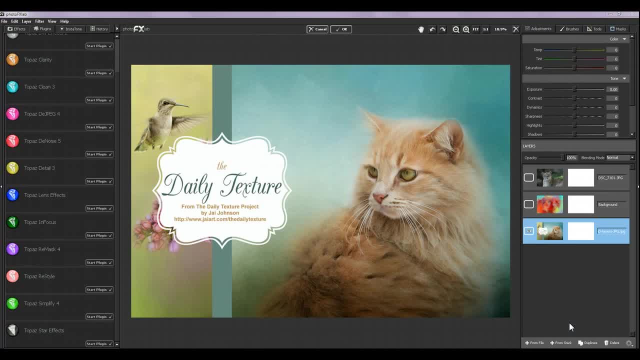 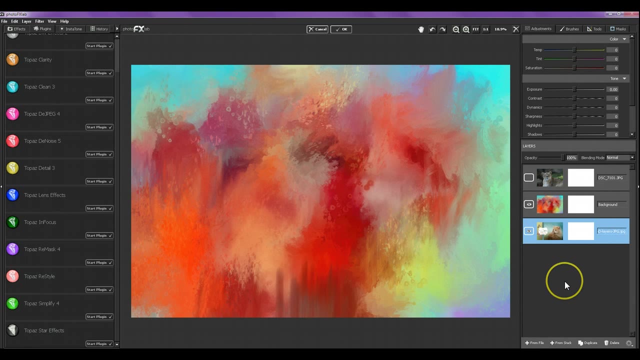 the same way, every image, and they've all worked very well. So I thought I would take you through number six, which I have not done yet, so you're watching this right as I'm doing it from scratch. Here is the texture. As you can see, it's very 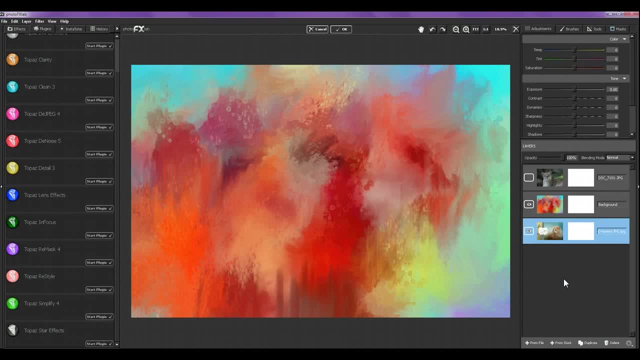 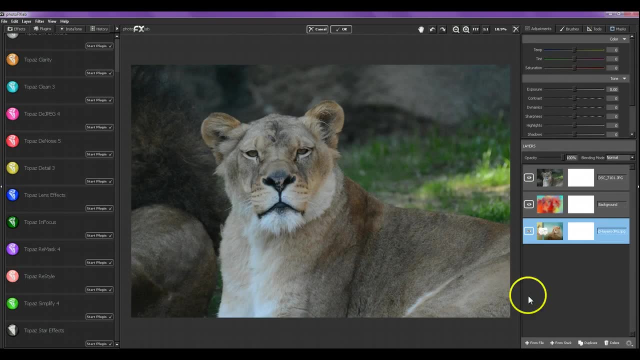 bold, very abstract, lots of color, very saturated, And I'm going to blend the texture with this photo of a female lion. I've done several male lions. I figured it was time for the female to have her time, So the first thing I'm going to do. this photo was: oh, let me back up just a second. I've 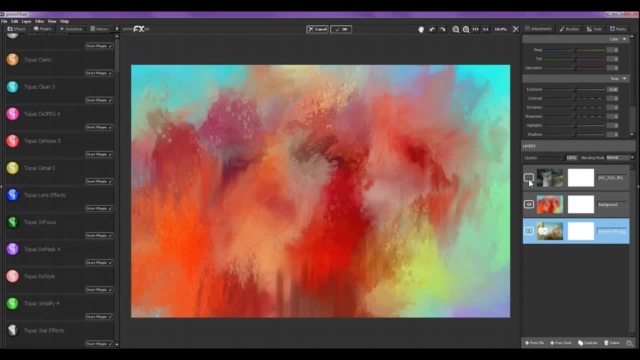 the textures are so bright. I've been using a lot of images that are taken in direct sun. This one has a little bit more of pastel colors through here and this is going to warm it up- the oranges and reds anyway- So I thought I 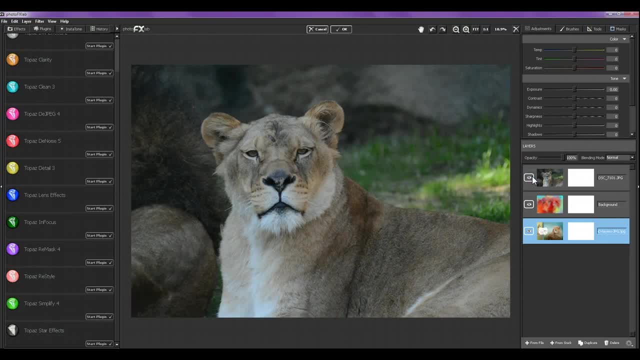 would try this one with a photo that was not taken in direct sun. So I chose the lion, because her colors are a little softer and I thought they might blend better with the pastel parts of the texture. But we'll see if it'll work, or 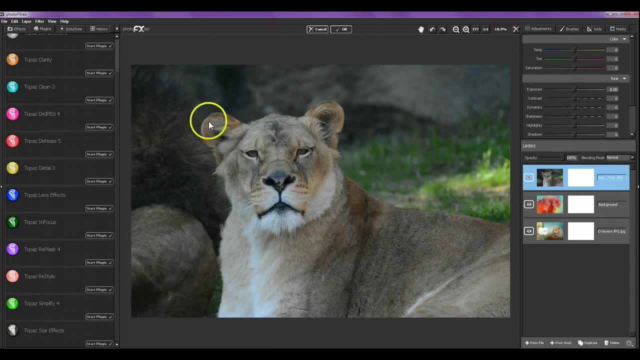 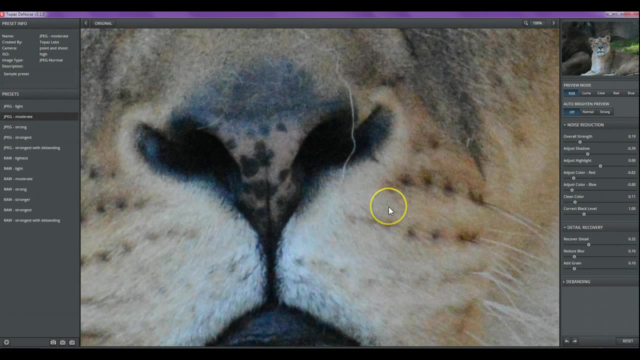 not First thing I'm going to do, because the photo was taken. this one was taken in a little bit of shade. there's a little bit of graininess here, so I'm going to denoise it And I'm working in Topaz, the Topaz software suite. Okay, there she's. 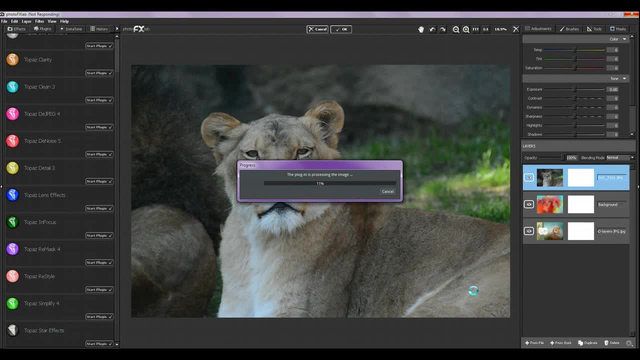 getting denoised now, just to take down that graininess a little bit, And this process just takes a minute. As many of you have watched my videos before know that I love Topaz, the software I log, I go into it. 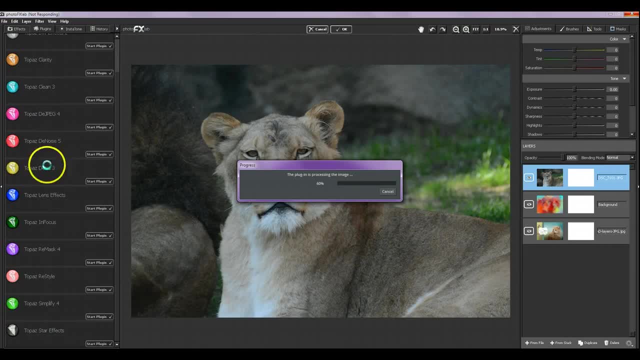 using the Photo FX lab filter, which gives me access over here to all of the different modules that I have purchased from Topaz, And I just like to go in there. that way, I can use whichever one I want. Okay, Miss Lion, I'm ready for you. 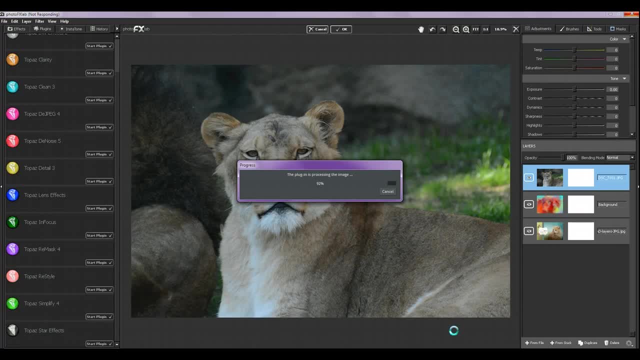 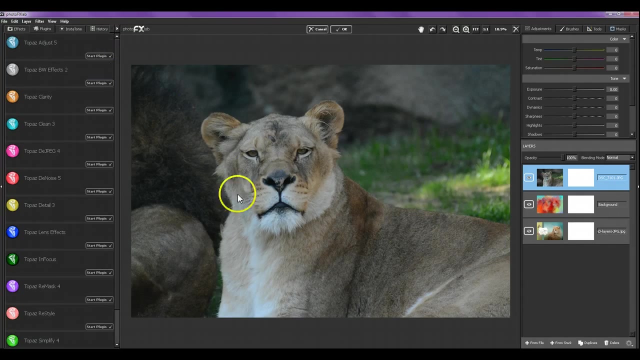 to get done. This is probably the slowest process of it right here, And she's almost there. Takes just a minute for it to register. Okay, she's denoised. Now what I've been doing with these is I really want to pump up the. 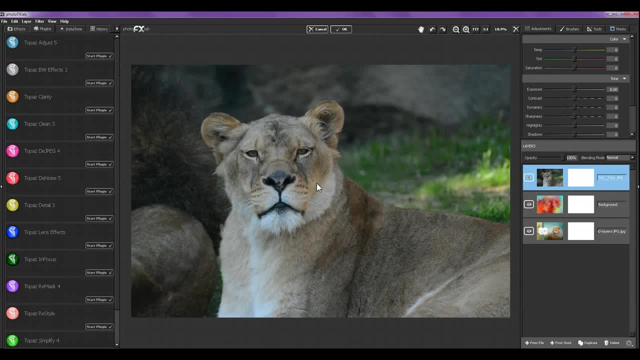 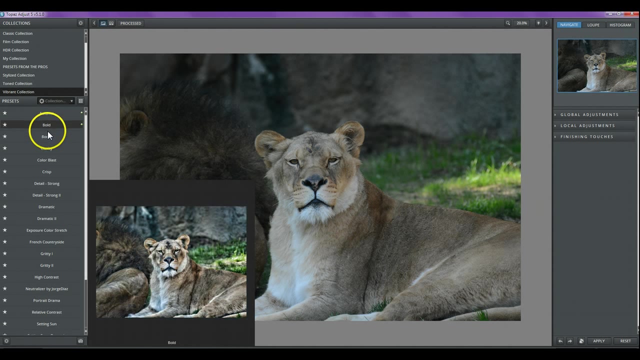 color And I pump up the detail and then I take some of the detail away And I'll explain that in a few minutes. So we're going to go into Topaz adjust and in the Vibrant collection. there's several choices here And I like to use Bold. 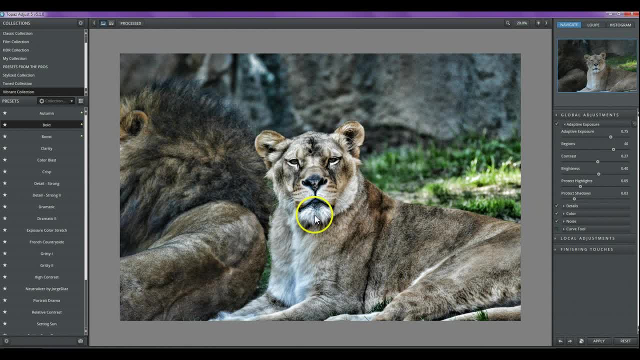 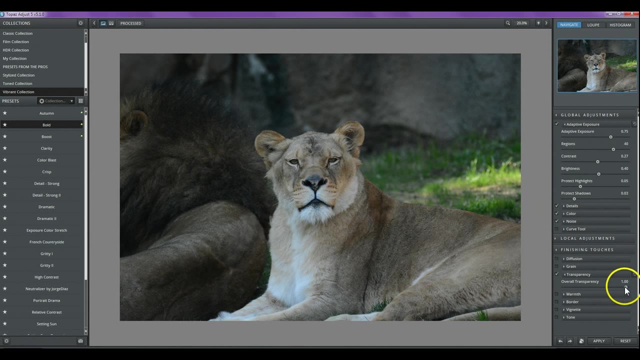 right here, which brings out the detail. However, I'm not sure if I think that's a little too much detail, So I'm going to choose the transparency. Right now it's set on zero transparency. If I bring it all the way over to the right, takes it. 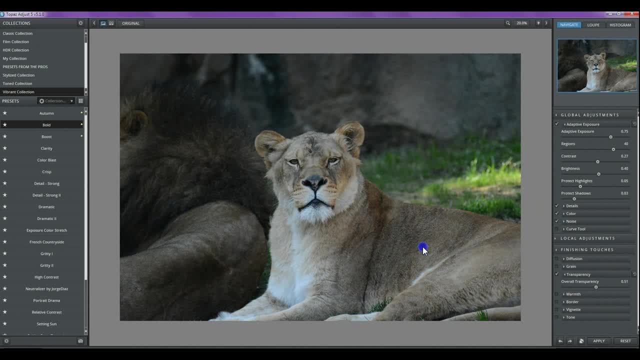 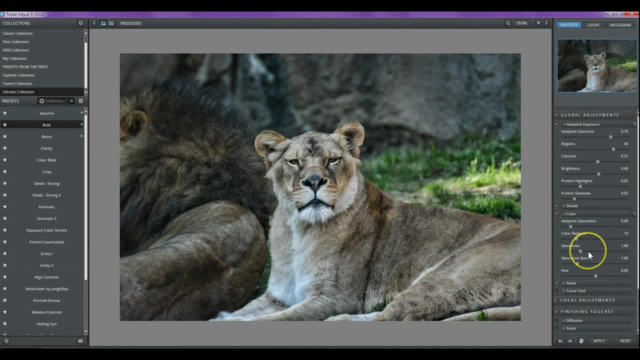 all away. I'm going to put it somewhere in the middle. It just pumps up the division of colors a little bit. I'm going to click on the color tab and see what I can do about boosting her saturation up a little bit. There we go. 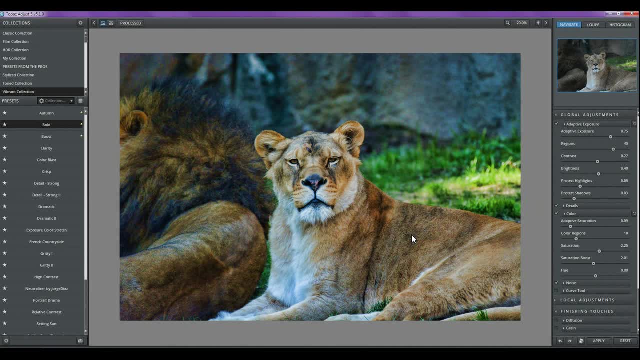 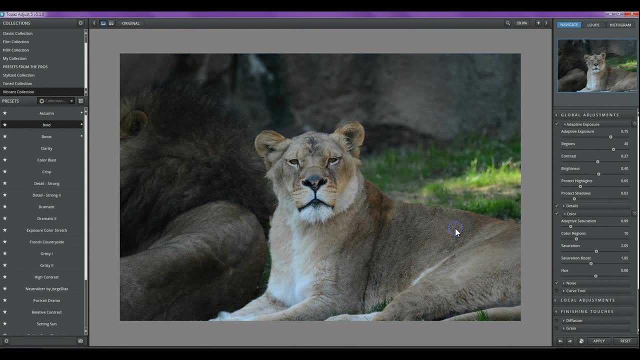 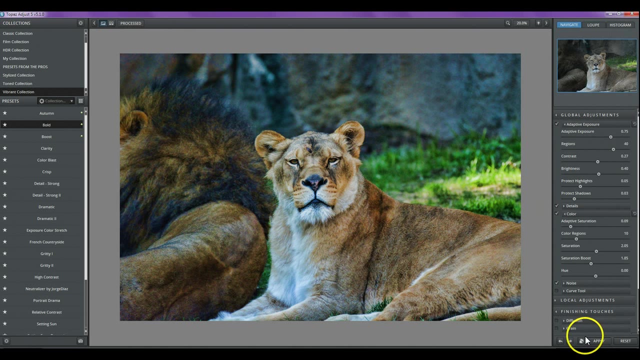 Because I, since the texture is really saturated, I want her to be really saturated as well. It may be a little too much. Okay, I'm liking that. So we're going to hit OK and let it process through this And I. 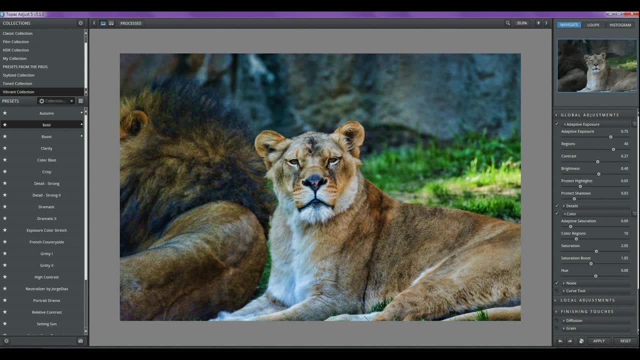 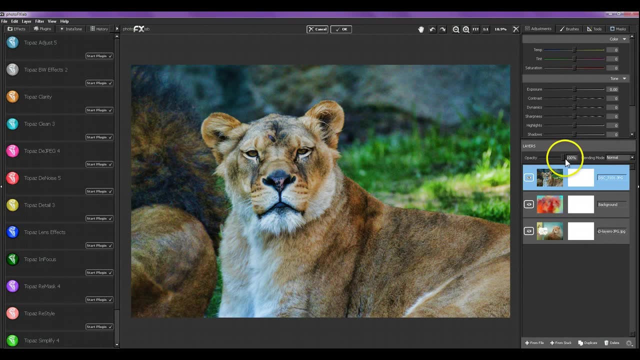 should have duplicated my photo layer, but I didn't. But that's okay, I can work with it. Okay, so now she's a lot more saturated And if I bring down her opacity a little bit, you could see how she's going to blend with this texture, which I 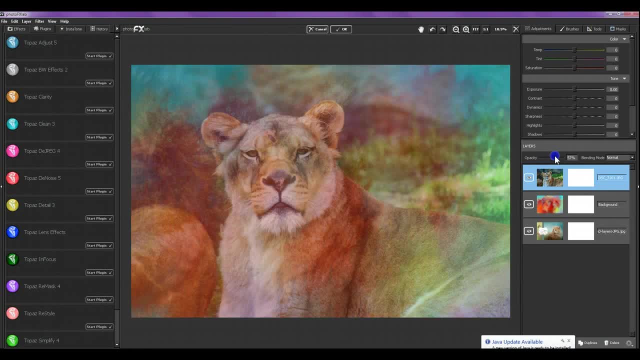 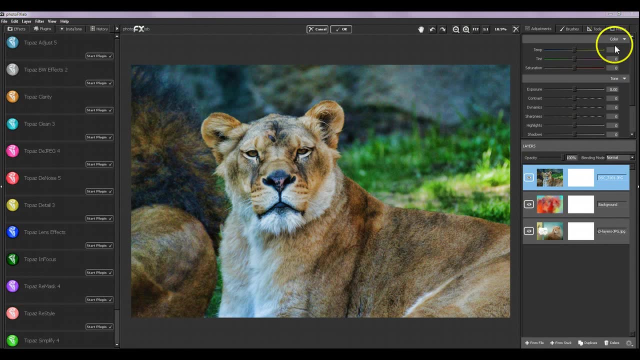 do this a lot, Just kind of move my opacity to see if it's going to look right and the reds and golds or oranges are in the right place. Now I'm going to mask away the background and actually bring the texture in with the line. So this is my masking tab. here I'm going to 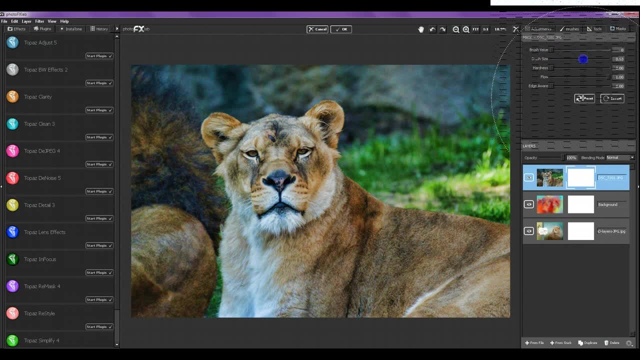 turn the flow all the way up because I want to get rid of all of this. I'm going to bring the brush size up and I keep the hardness on the brush right here. I keep it all the way down. I like a very soft brush. 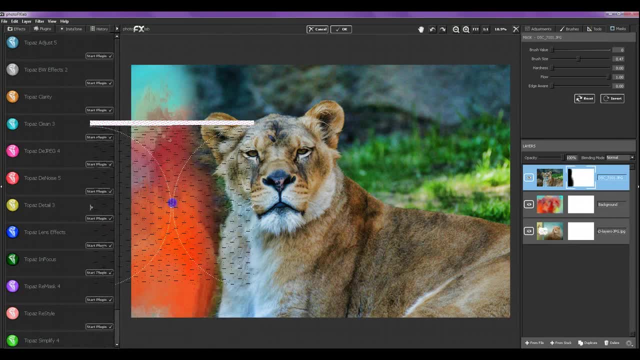 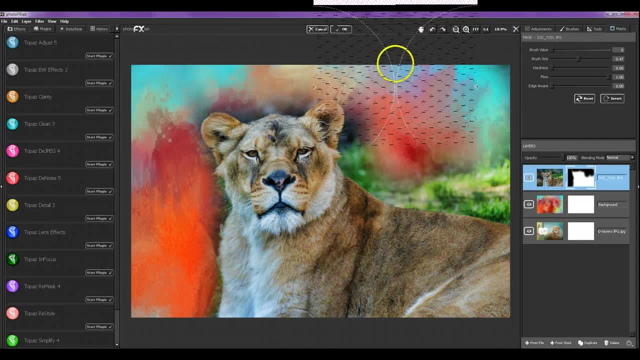 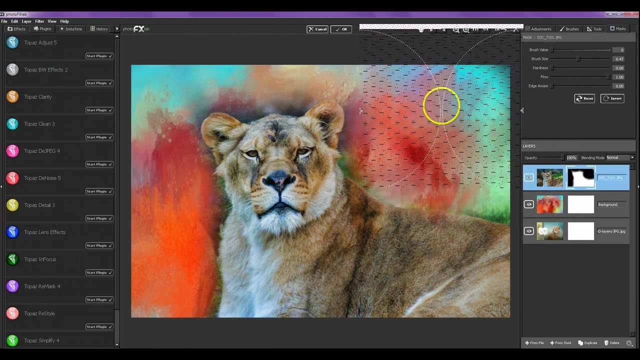 And I'm just going to go around the edges, getting close to her but not coming over her fur at this point. Now I could use Topaz Remask if I wanted to get a very exact mask around her, but I don't. This is an abstract texture. I'm trying. 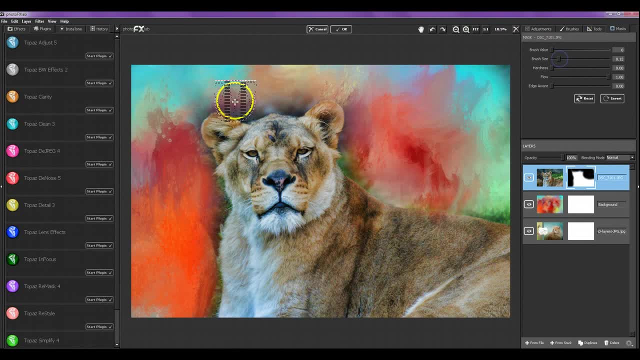 to create an abstract work of art. I'm not worried about perfection Now. I lowered my brush size here so I can get in closer- around her ears, top of her head, And I'm basically masking this totally away at full opacity. so it's bringing. 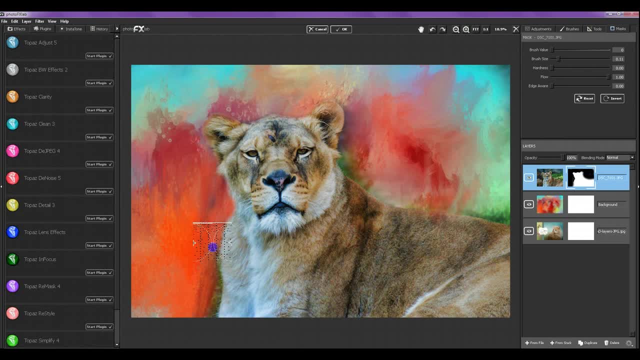 the full opacity of the texture through, And I'm just going to go as close to her edges. Oops, Control Z is your friend when you make a mistake. And I'm going to go as close to her edges as I can without going over her fur. yet I may go over a little. 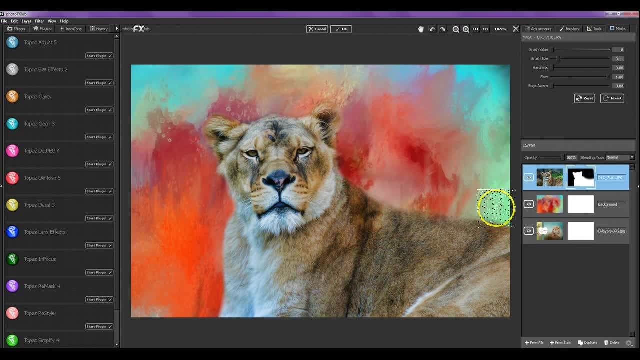 bit, but I can always fix that later if I want to. Now you could see the little mask here and I could see some little areas on this side here and across the top that aren't totally black. So I'm going to look, looking. 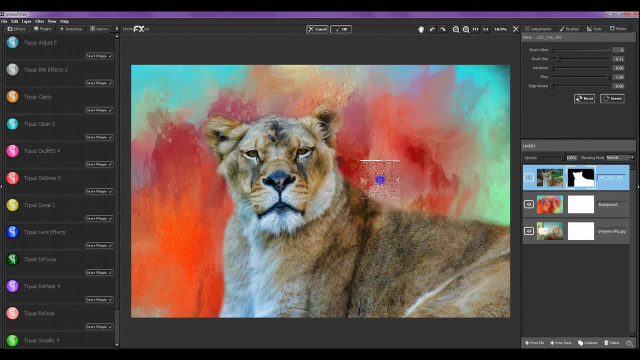 at my mask and then go over here to try to find those spots like this corner right here. You can see how it changed that. And then I'm going to make the brush big and go over that again. case I missed anything, I'm gonna make it smaller. come right around the top of her. 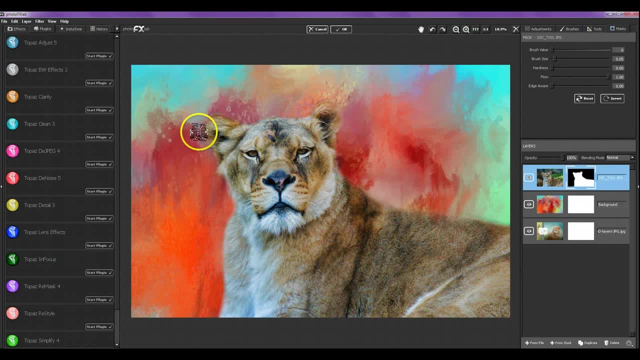 head here where there's this black showing, because I want this to blend right here. okay, now I've brought the texture in as the background. now I'm going to bring some of the texture over her fur. so at this point I'm gonna lower the flow, which is like opacity, make the brush size a little bigger and just kind. 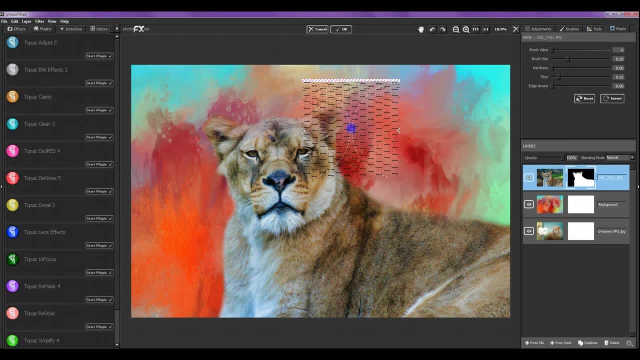 of gently tap, very short strokes as I bring it over her fur, just to get an idea of how this is gonna look. I'm gonna go all around her edges and then down here in this corner and even across the bottom, just a little bit. now I'm gonna. 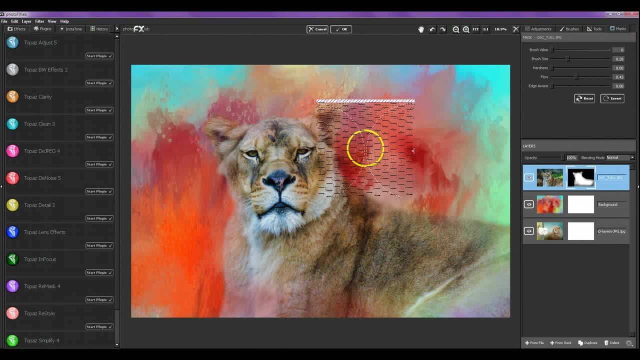 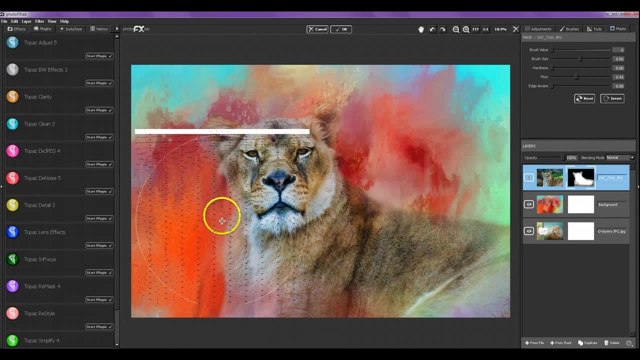 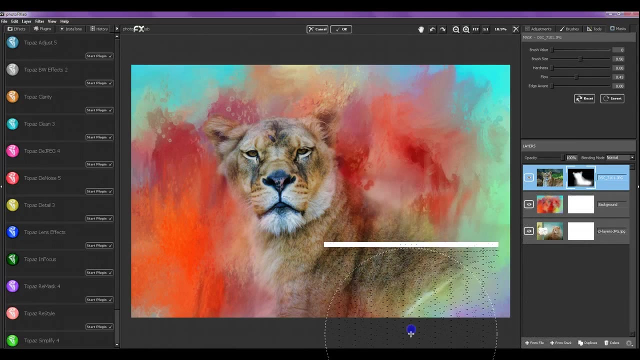 brace the flow up, which is gonna give me a stronger shape, masking away of the texture. I'm gonna bring the brush up and, just to see how this is gonna look, I'm gonna bring some really strong texture over her with these very strong textures. don't be afraid to just really bring it over the. 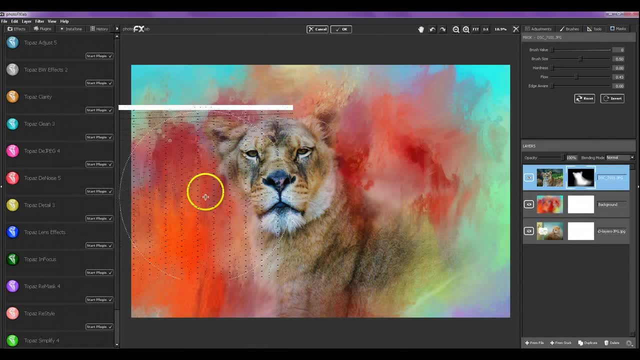 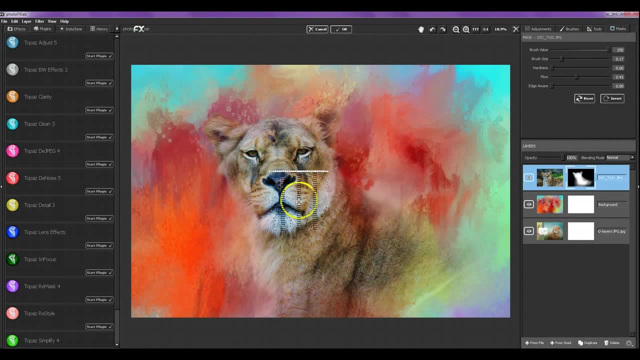 subject and just see how it's gonna look now. I've masked away a little bit too much of her, so we're gonna lower the brush, put the brush value to the other side, which will reveal some of this. bring some of this back to the other side. 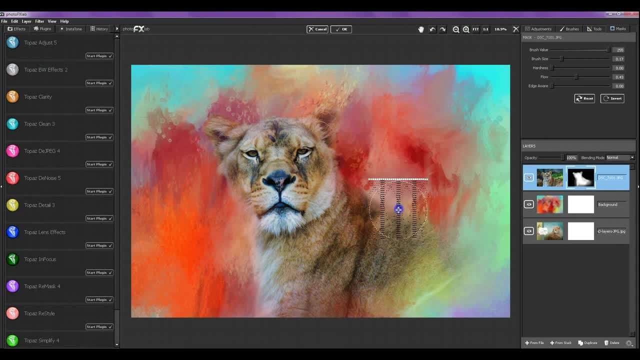 back. let's say here: okay, that's too much. ctrl Z because I want- I don't want any of her background showing and we'll lower this flow a little bit. make the brush size a little bigger and just tap through here to reveal just a little bit. 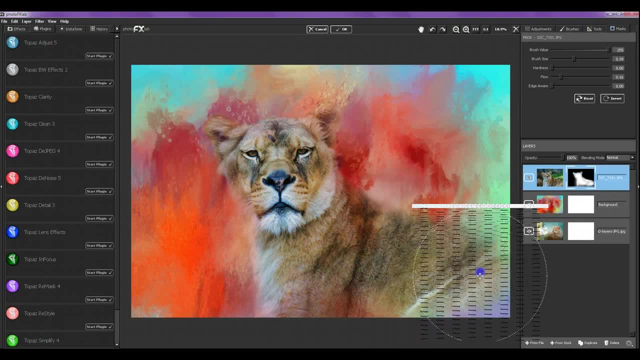 more of her body, right there, her leg, and I still think I want some more of her back. let's see here- okay, that's too much- ctrl z because I want- I don't want any of her background showing and we'll lower this flow a little bit, make the brush size a little bigger and just tap through here to reveal just a little bit more of her body, right there, her leg, and I still think I want some more. 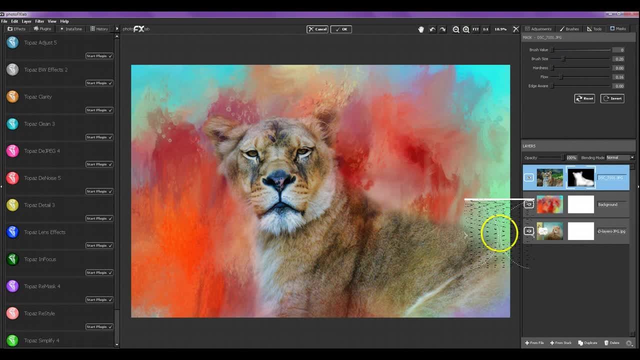 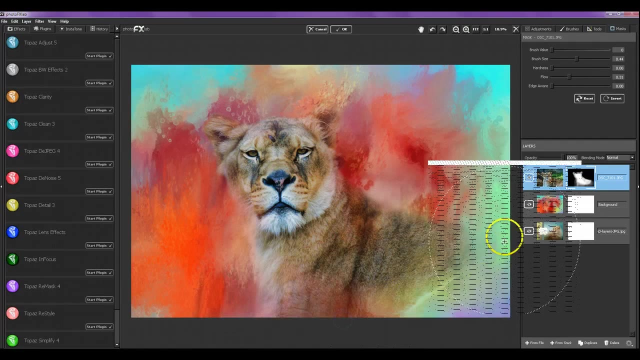 texture brought over that corner. so I'm gonna make the brush a little bigger, make the flow a little bit more and just kind of gently sweep around the corner, sort of creating a vignette of the texture, and then around here too, and then- and this is how I do, back and forth, back and forth- I get a little too much. 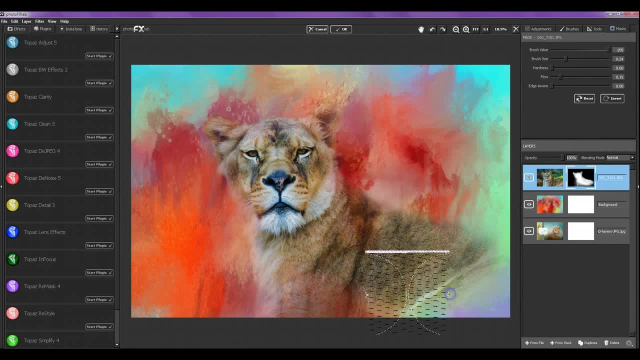 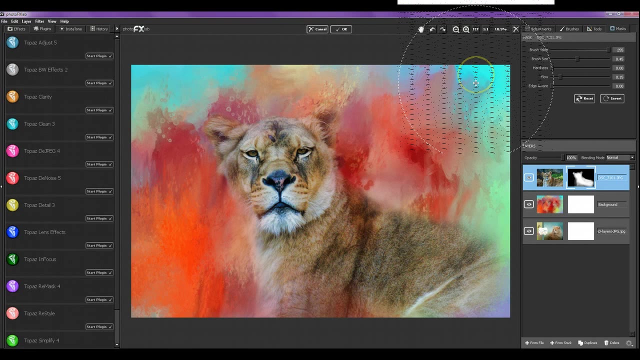 I'll back some of it off and I adjust the flow constantly and tap, I tap quite a bit, but that brings the texture right into her and that's. I'm kind of liking the way that looks. now we're going to do some other things which are going to. 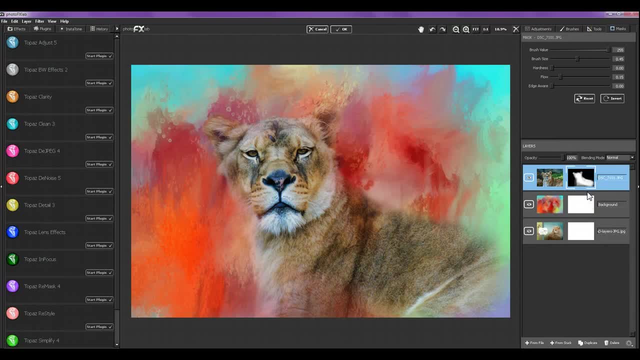 change this even more at this point. here's what I've got. I've got a very simple abstract. let me lower this brush size because it's too big. it's driving me crazy all through here. it's a very abstract texture. and then I've got a. 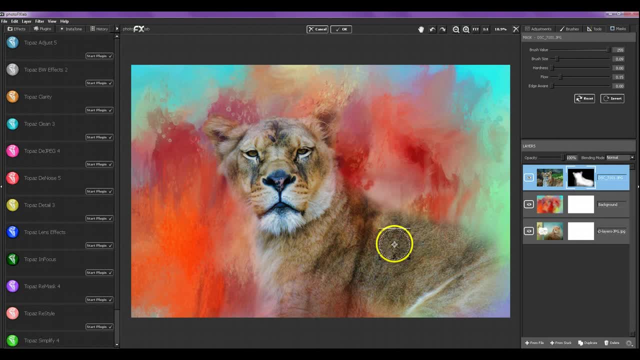 very realistic lion because it's a photograph, so it's going to be realistic. mask some of that off right there and some of her ear. keep her ear showing a little bit more the. when I first started doing these, I would get to this stage and I would think, well, that looks okay, but there's something wrong with this. 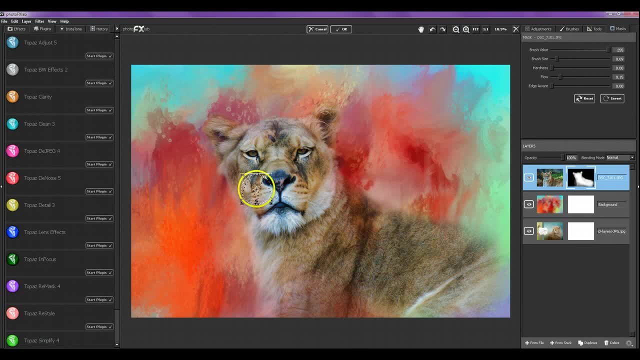 picture. there's something I'm not liking about it and what I realized was this texture is very abstract, very painterly, but this is not the. the subject photo is too realistic. so at this point is when I started playing with some filters to give the photo a more painterly look. so this is what I'm going to do. I'm going 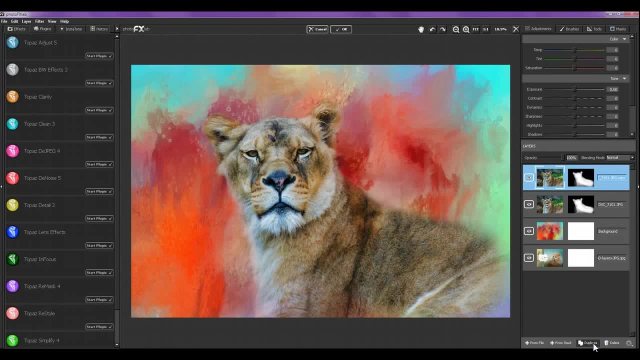 to duplicate the photo layer, which is going to be the layer that I'm going to make her look stronger. so you see the difference along. look like watch right here when I turn that duplicate layer back on, right in through here. it makes the edges, brings back some of the edges I've masked away and makes them stronger. 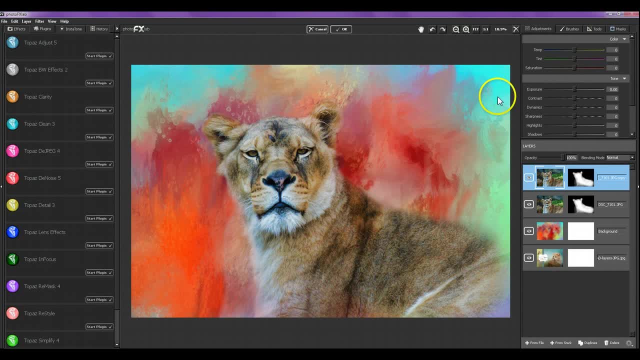 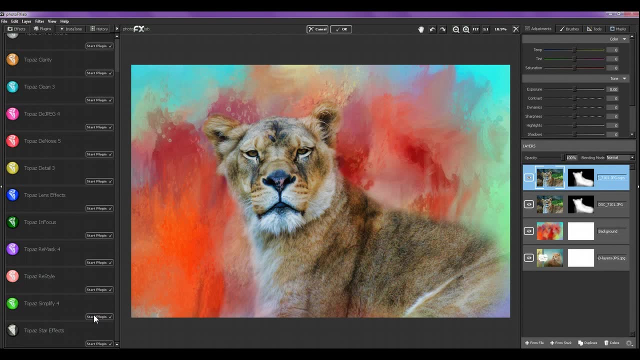 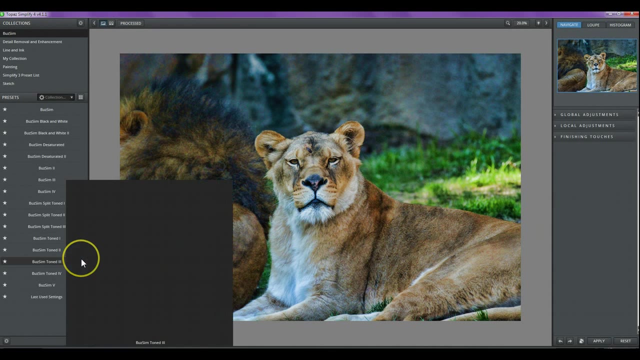 see. now that's fine, except for she needs to get painterly. so I'm going to go to topaz simplify, which is where the painterly filters are, and I have two favorites. I have one called buzz sim that I try, and I also have the pastel that I like. we're gonna try buzz sim first, we're gonna click. 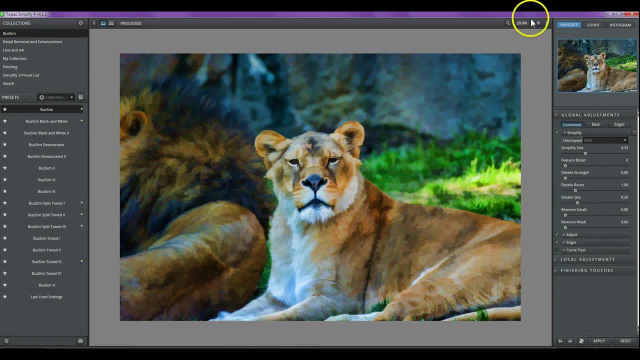 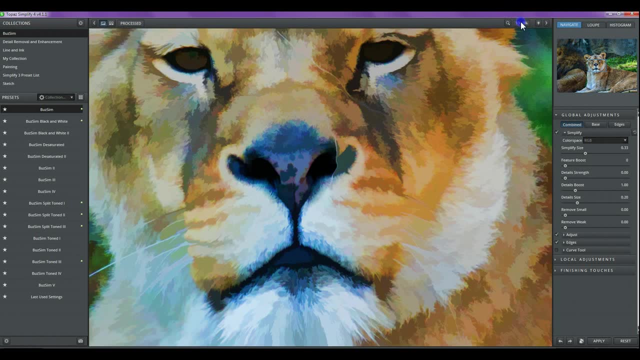 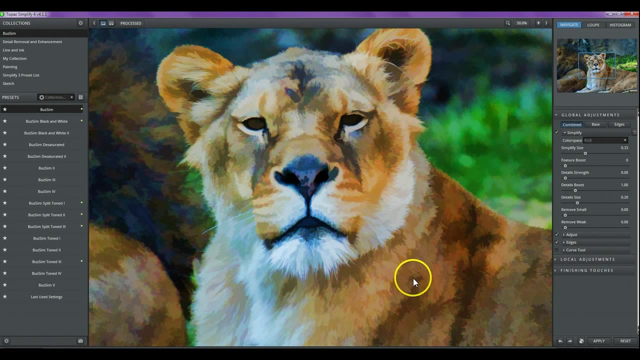 that now she's looking kind of painterly. let's. my goal is her face, though, so let me raise this up there now. you can see it's made her look very painterly, but it's a little different. now I'm going to go ahead and make her look more. 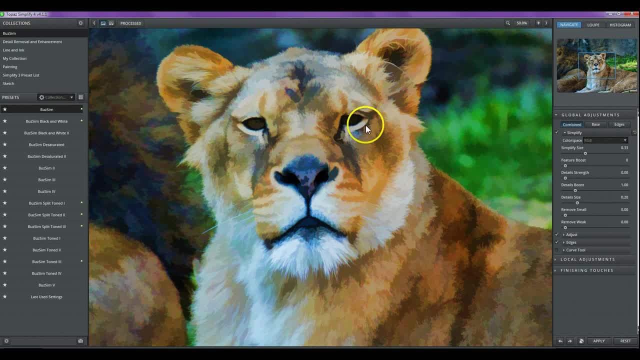 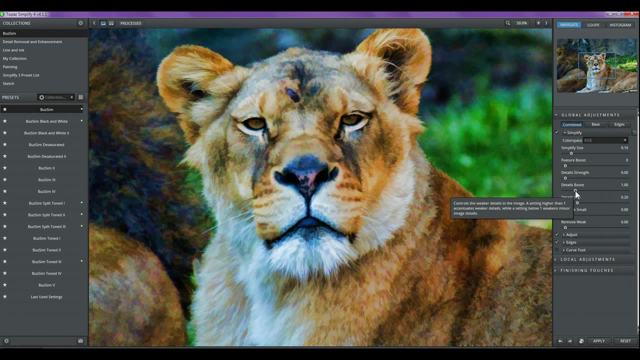 choppy I. it's a little bit too much detail lost, so I'm going to reduce the size, simplify, size down, which is going to bring back some of the detail, and I play with these settings in here. we really don't need a lot of details and I. 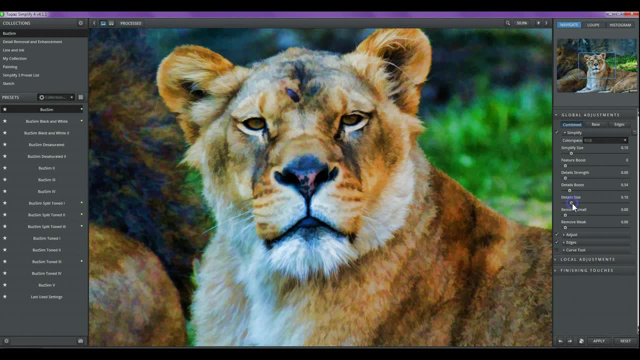 turn them down and up and just mess around with them um, back and forth. if I screw it it'll just never alter anything, but that's fine. until I get done with it up, I always hit the reset button. Let me see, here I am going to boost her saturation just a little bit. more. Structure Now this. 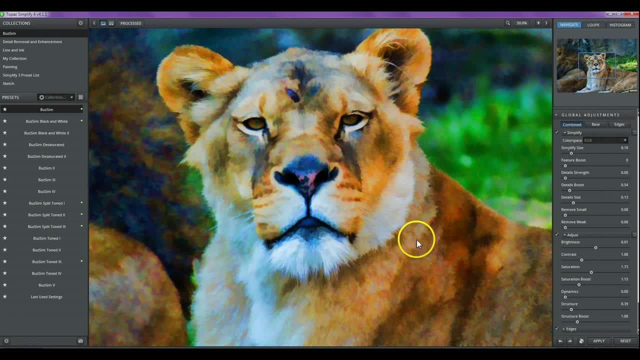 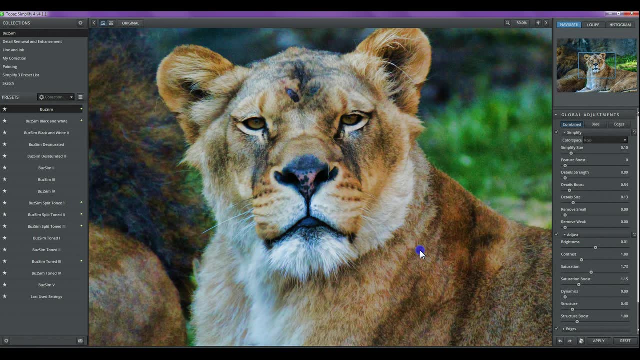 might help to take there we go now. see, that takes those sharp edges down a little bit, Because I don't like the sharp edges of the painterly. look, This is the original and this is what I've done. So now it looks more painterly and 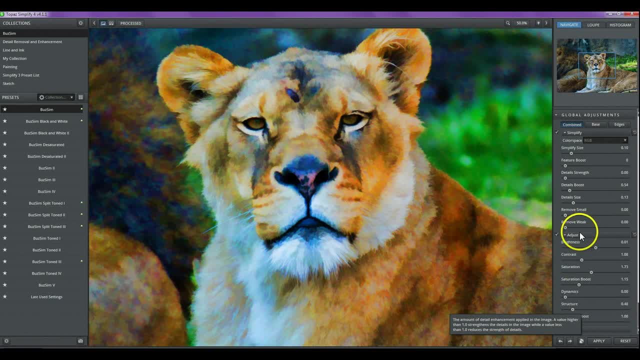 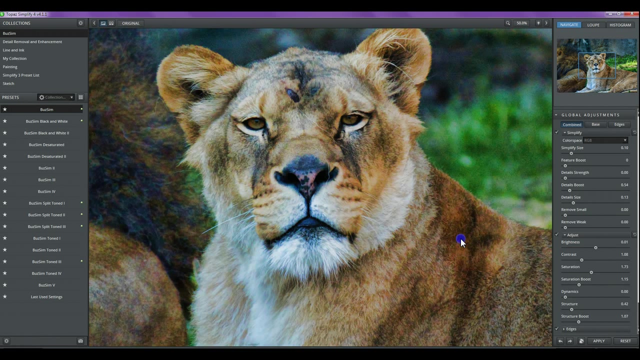 I've reduced the sharp edges by going under the adjust tab for this particular filter and going to structure and taking that down, And I'm going to take the structure boost down just a little bit and maybe raise the structure up a little. I like the structure boost up, so I'm going to put that back. Okay, that's the. 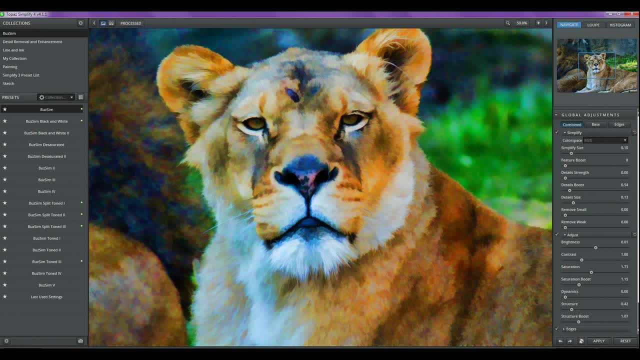 photo. This is the painterly look. Now we're going to hit ok and let this process, So this is on a separate layer because I've duplicated my photo layer. After this gets done processing, what I'm going to do is go on this layer, the 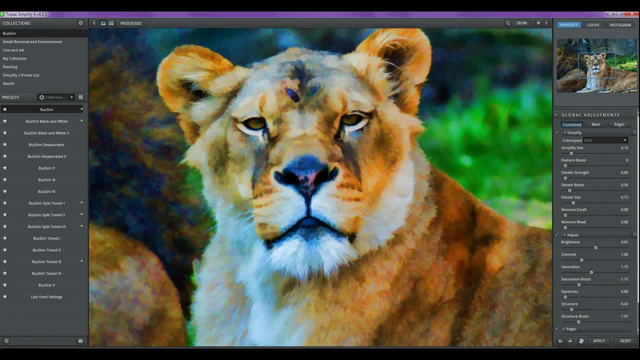 painted layer. I'm going to mask away some of the eyes and the nose and the mouth a little bit to reveal part of the photo underneath. I'm not going to do very strong masking away, just to bring a little bit more detail back through here. so it basically ends up being a mix of a painting and a photo which, when blended, 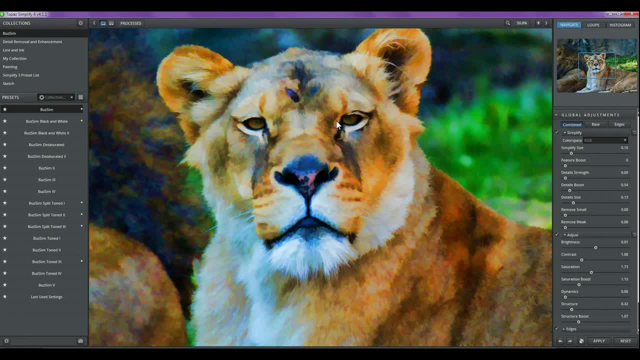 with the textures make a very nice finish. look, you're gonna have people say: is that a painting or is that a photo? and you're gonna say yes, because it's both. now you can use any painting filter that you would choose in any of your software. I know a lot of softwares have different filters. I know there's topaz. 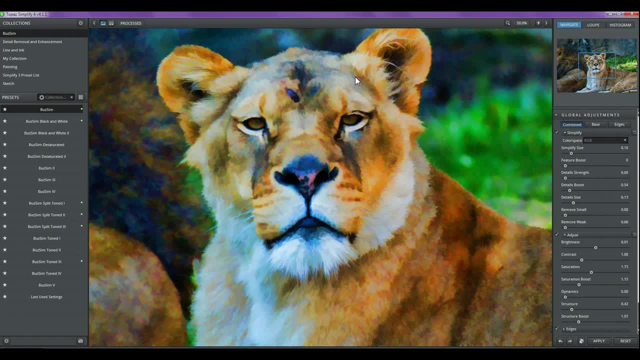 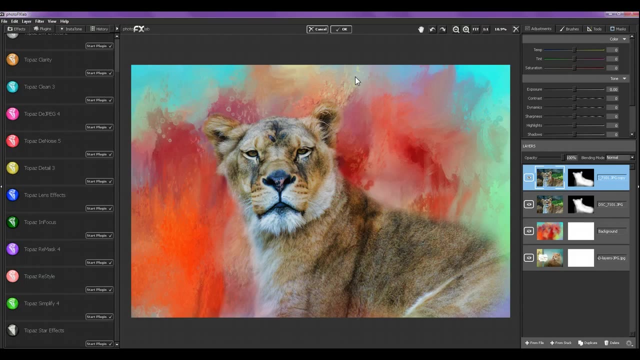 impressions, where you could pre make a layered of the photo that you're gonna work with as a impression- mystic painting- and then put it on top of the original photo and mask parts of it away. so watch my photo here as it becomes very painterly. there we go now. 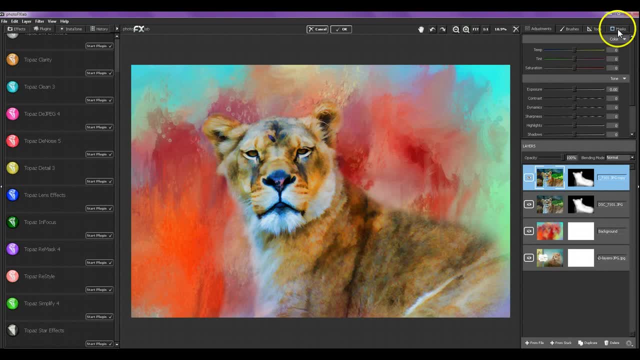 that this is where I'm gonna mask away some of these eyes. so we're gonna go back to the mask and leave the flow down pretty low, brush size, pretty small, and I'm just gonna go in here and gently mask away some of the patterns that I just made. it's a little tricky. sometimes you just want to paint. 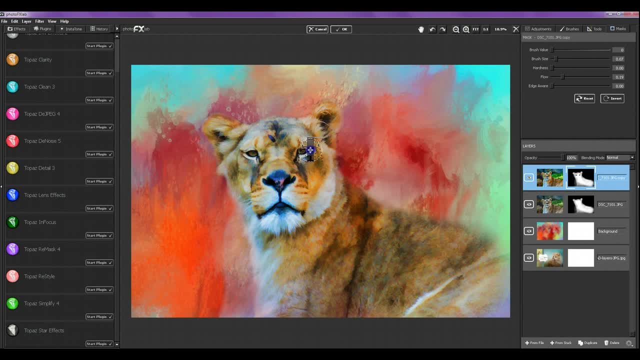 them like that. the only possible way to do that is to start a new painting, is to painted part of the eyes, which will reveal a little bit more detail. I'm going to do the same thing around the nose area a little bit and bring back some of the nose and mouth. 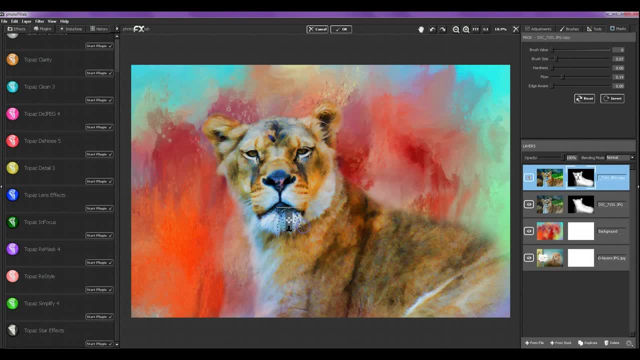 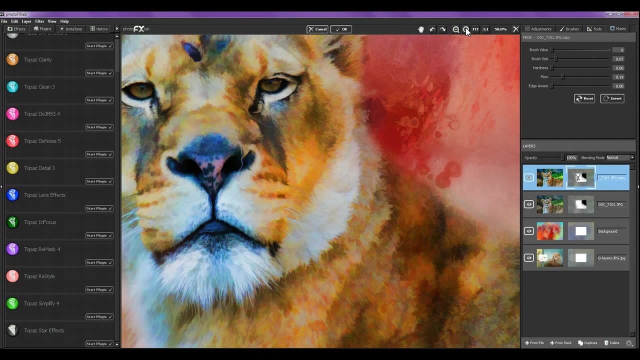 detail and a little bit of the fur here around her mouth. There's a little piece of fur, loose fur, hanging over her nose, so I'm going to get that and a little bit of ear fur just to reveal some detail, and I'm going to blow this up so you can see. So see now her eyes. 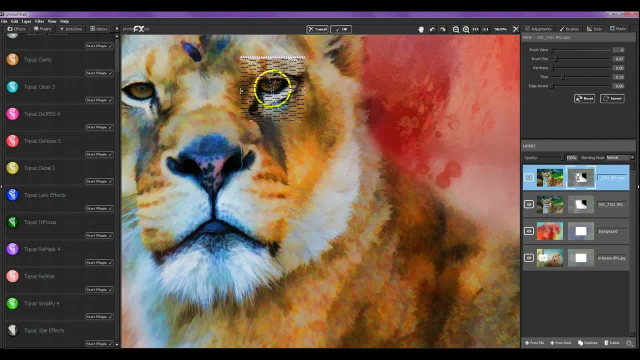 look or part of that is masked away, revealing the photo of the eyes underneath and same with the nose and some of the fur, but most of it I'm leaving painterly: The eyes, nose, face, mouth. all of that is the most important part. 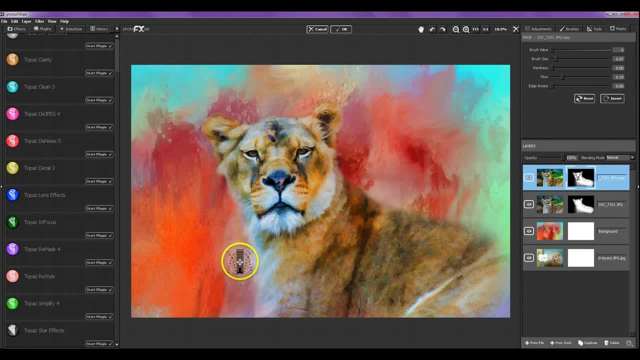 Okay, Okay, Okay. Now, right here. I'm not liking this. If I turn this layer I just did on and off, that is making that look a little bit less. I'm going to go back to the original photo layer, back to the mask. 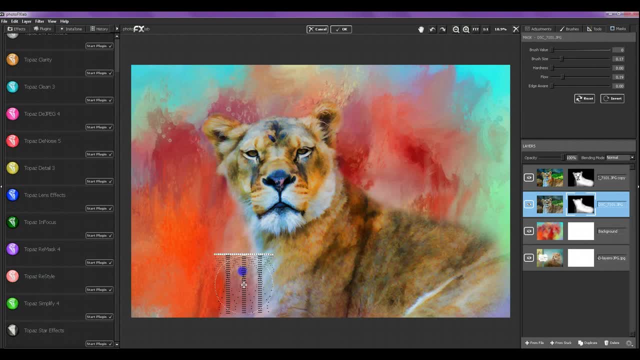 and I'm going to remove some of that texture from that portion of her right there, Because that's actually her. well, I'm not removing it, I'm putting it back on. No wonder it's not working. See, I told you I was doing this from scratch. You're just kind of along. 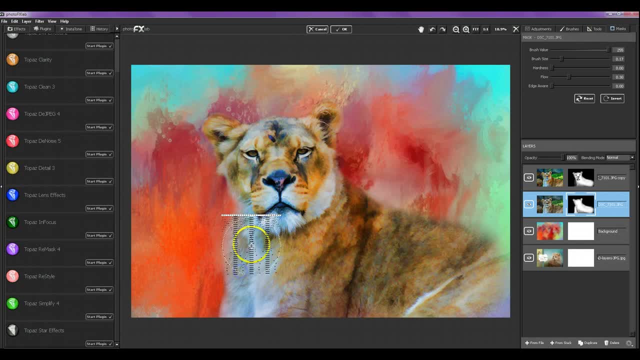 for the ride here. Okay, Now that's revealing more of the fur. I might actually try to reveal a little background here. let's see how that'll look. I still need to pull some texture back over there, so we're gonna go back the. 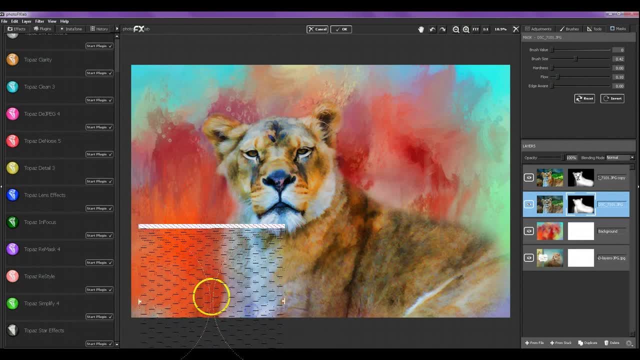 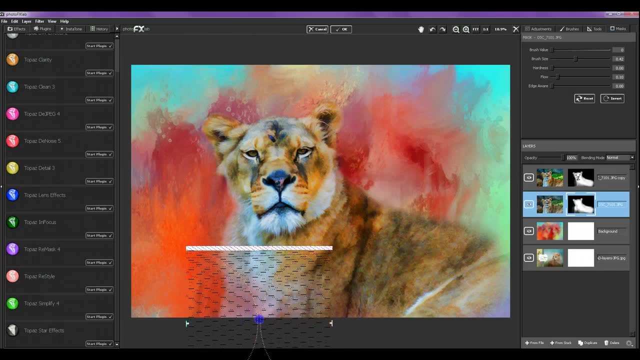 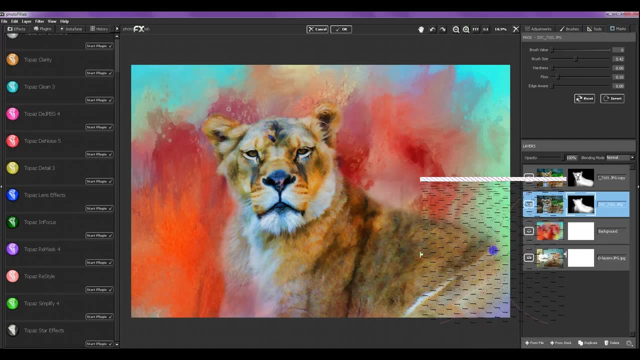 other way and we're gonna come down here right along the bottom of this leg and just kind of gently brush- I'm using a very soft brush and a very low opacity- and tapping, and then back to this corner again. This, these corners, really. 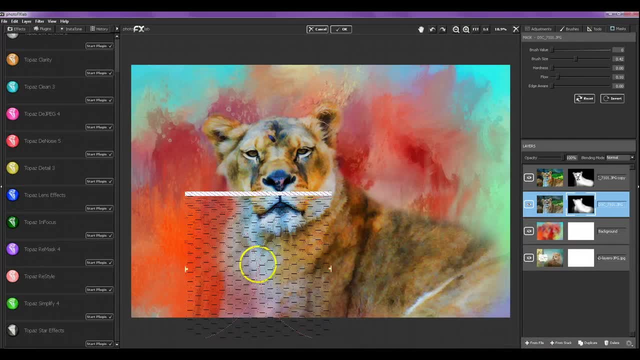 bug me. I like them to blend fairly smoothly, and this ear is bothering me up here, so I'm gonna reduce the brush size and actually work on coming over that ear a little bit more And bring some of that texture right down over her fur, right there, It's just. 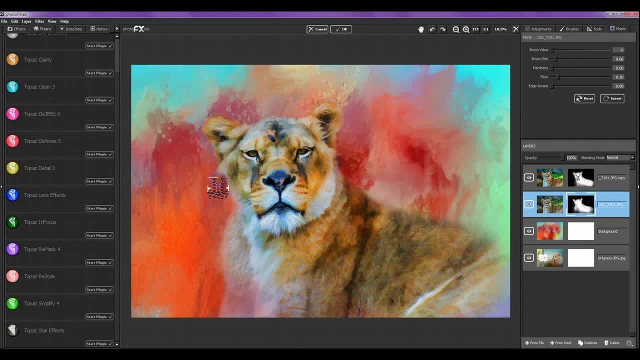 like painting. You're just painting away her fur, or painting her fur back and revealing the texture that's underneath, And just go around her a little bit more. I don't like sharp edges. I like everything to blend. Now, that's looking. 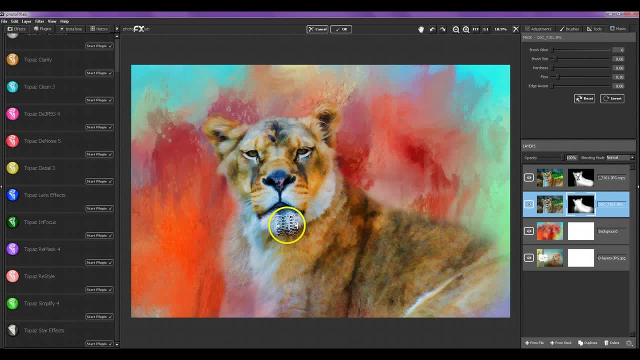 pretty good. The problem is she's a little bit got a little bit of blue cast here Okay In her fur, which I'm not liking. So I'm gonna see if I can fix that And I'm gonna try to fix it on the painterly layer. I'm gonna go back to Topaz Adjust. 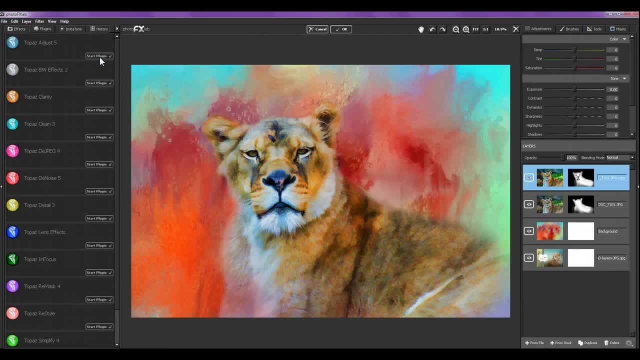 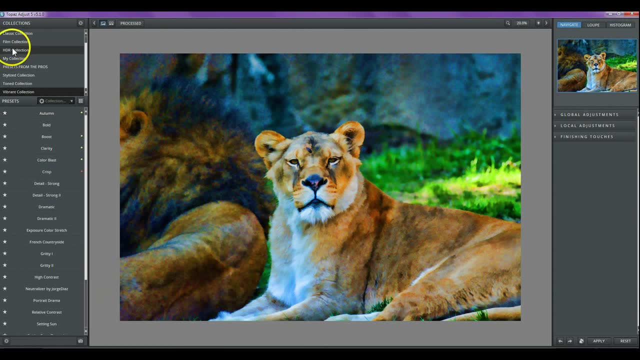 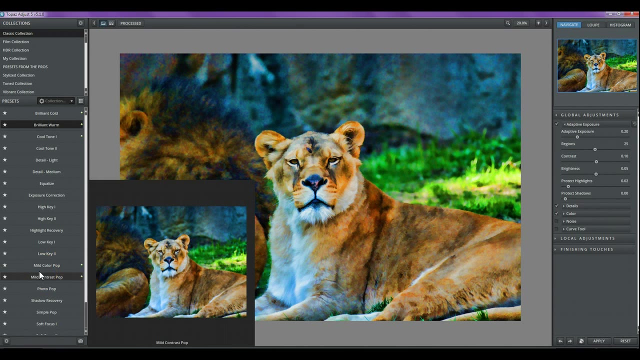 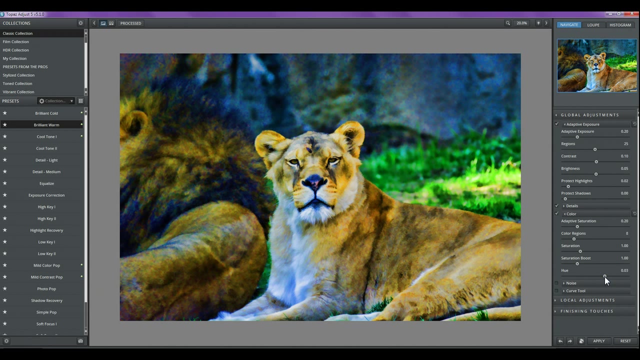 and see if I can do something to warm up that the whites there, Because they're a little bit too blue. We're gonna go to the classic collection and try Brilliant Warm. Now that didn't work. Um No, I don't like that either. That made her a little warmer, Too warm, And reset. 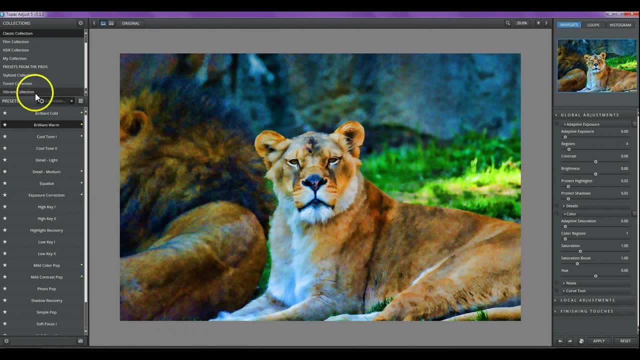 This is when reset comes in handy. Let's go to the Vibrant Collection and try Autumn. Autumn warmed everything up a little bit, Including the blues, Just a little bit on. that's before the autumn adjustment and that's after, maybe a little bit too. 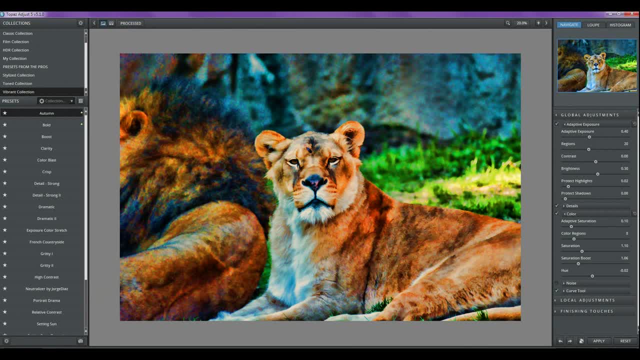 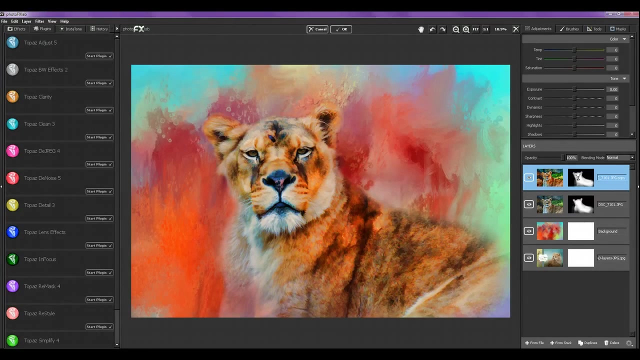 much. but that's where control Z comes in handy. we're gonna hit OK and see what this looks like. if I don't like it, I can control Z it and undo it. whoo, I like that. that made her fit in better with these oranges, the oranges. 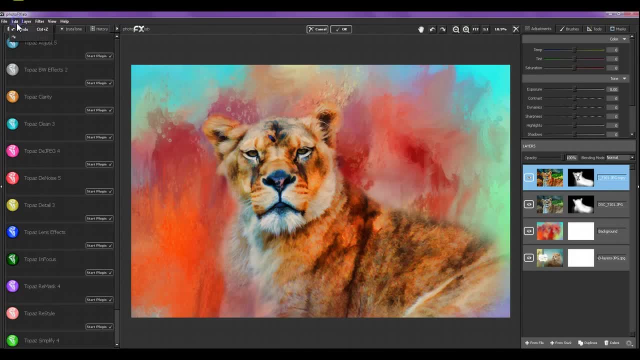 and reds here around her. let's undo it so you can see the previous one undo. see she's got kind of a greenish bluish cast to her, but yet this is really warm right here, which the greenish blue does fine coming in through here with these green 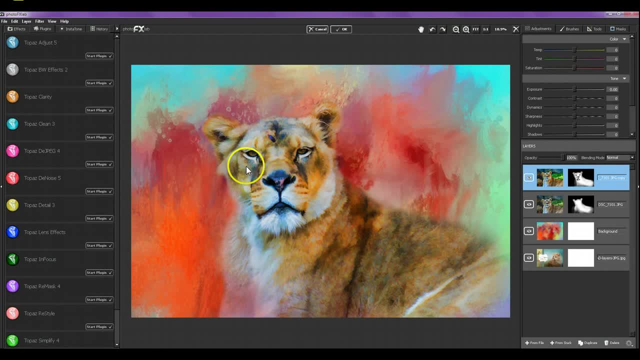 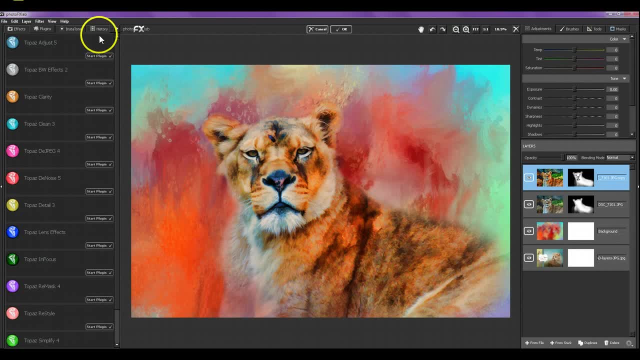 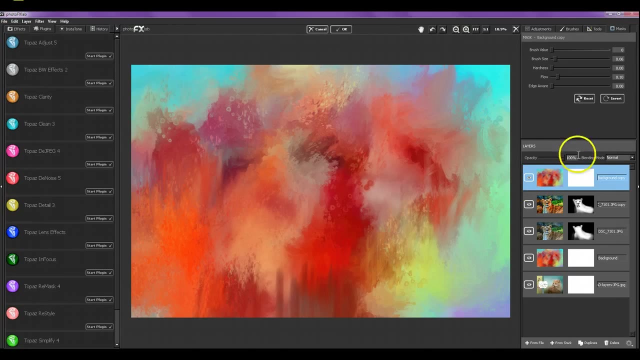 blends better with these oranges and reds right here. okay, I like that. now we're gonna play with actually duplicating the texture layer and putting it on top, and we're gonna play with some adjustments here, one of the ones I've been using with these particular images that are very 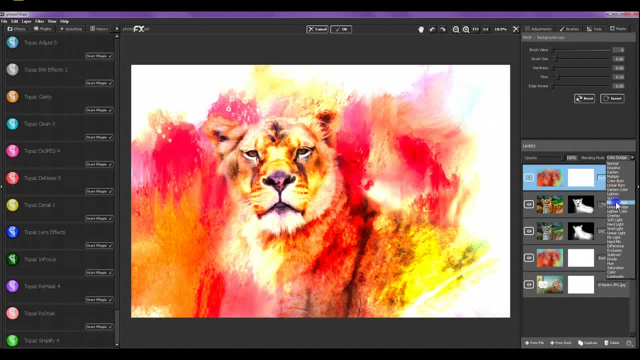 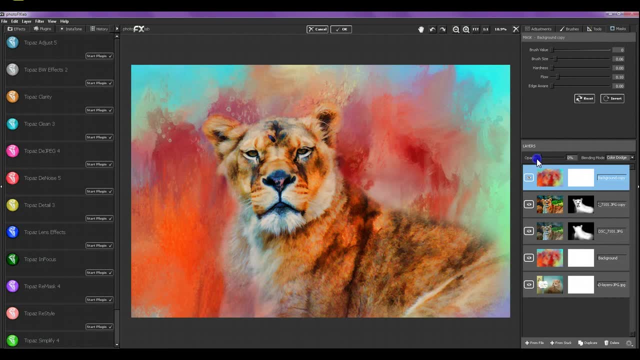 saturated with color is color dodge and that's full strength and that's very, very wild. we're gonna bring the opacity of that layer down to about somewhere between between 10 and 20. before-after still little bright, but I'm gonna leave it at 20 right now cuz I'm 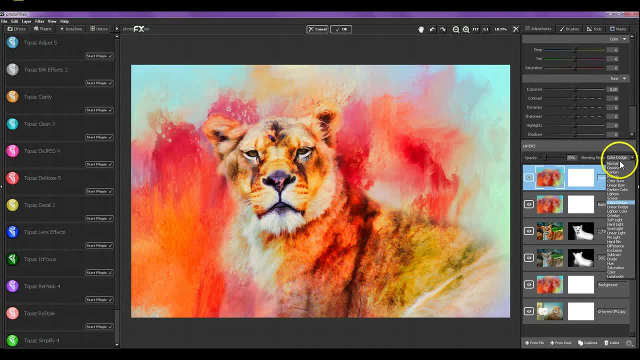 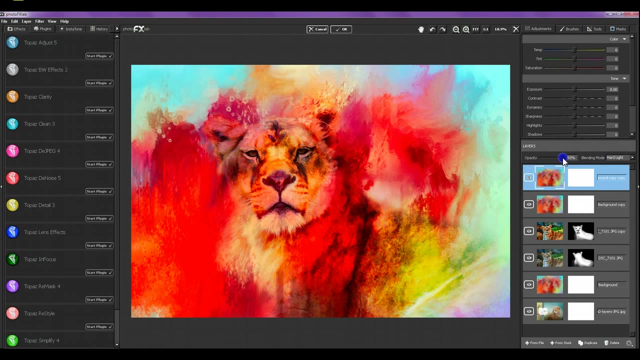 going to duplicate the texture layer again. I'm going to play with some other layer modes: Multiply, Overlay, Soft Light, Hard Light- Those are my favorites. Color Burn Overlay, Soft Light, Hard Light- Let's mess with Hard Light. Okay, Hard Light, let's. 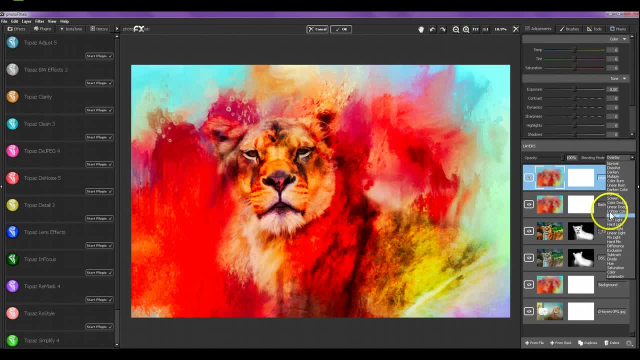 go to 100% and see what kind of adjustment we're getting. Multiply would make it too dark. Overlay is too saturated. Soft Light- okay, Hard Light is too much, Let's go to Soft Light but then bring that opacity. 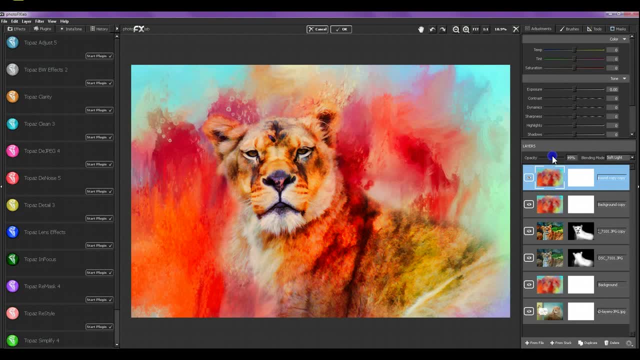 All the way down and then gently ease it up. 49 might be a little much. Let's try around 30.. Off, on, off, on, off, on, and I'll do that a lot. Now let's go back to the color dodge layer, take it all the way down and just bring it. 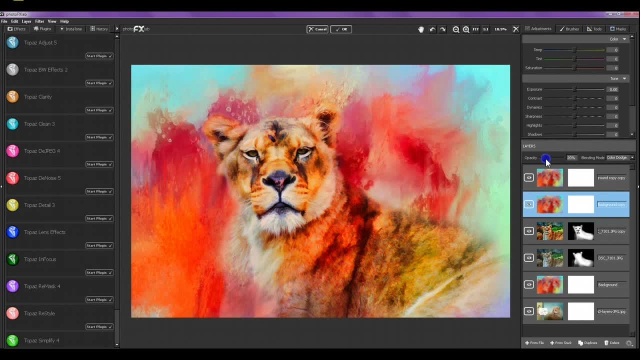 up very slowly until it's just a little bit brighter. I think 20's too much. I'm going to try 10. that's off and that's on. that brightens it just enough. I'm I am liking this. I think this fits really well. the only part that I'm not thrilled with. 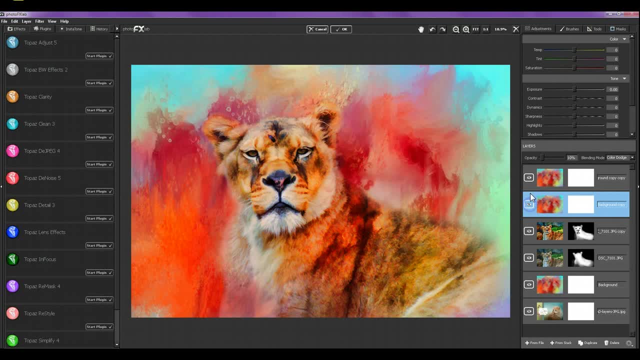 still is this right here? and I'm gonna tell you, I turn off and on my layers on and off frequently to see where I'm getting this from. this is coming from. that's on, that's off. when you turn the painted layer off, you can see this has a. 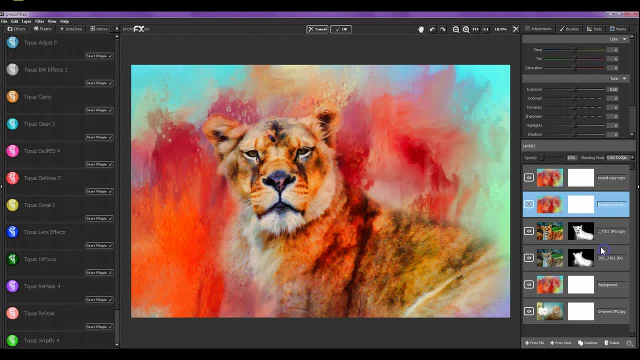 lot too much texture right there. that's coming from the original photo layer, so we're going back to that, back to a mask. we're gonna take off some of this right here again and I'll do this throughout. as I put those other layers of texture on top. it'll often reveal areas I'm not happy with. that's a. 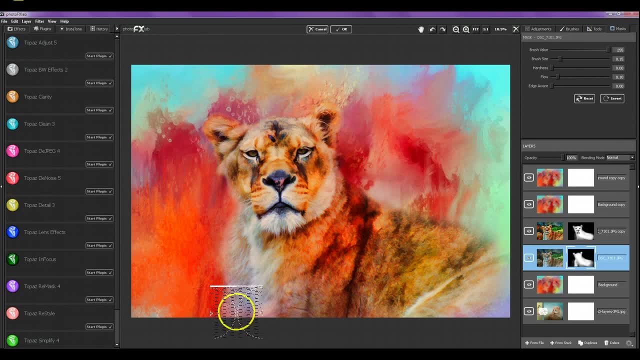 little better right through there. I could still bring a little of it over her leg. so I think I'll do that, but make a smaller brush and just kind of get rid of that hard edge right there. that's a little better than it was now. this is what I like to do. when I'm getting close to being done, I will zoom. 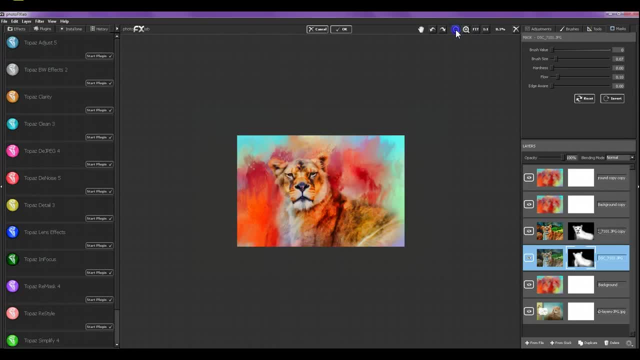 out on the image so I can pretend I'm looking at it from a distance, because a lot of times when you do that you can. you can close your eyes for a second, open your eyes and you can see your problem areas. I still think this bottom is a problem area. so we're going to have to do that and I'm going to put on some. 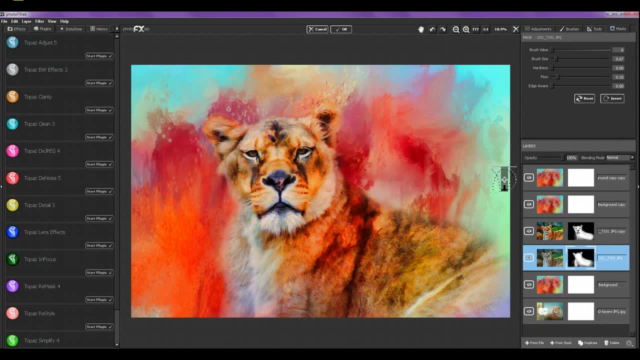 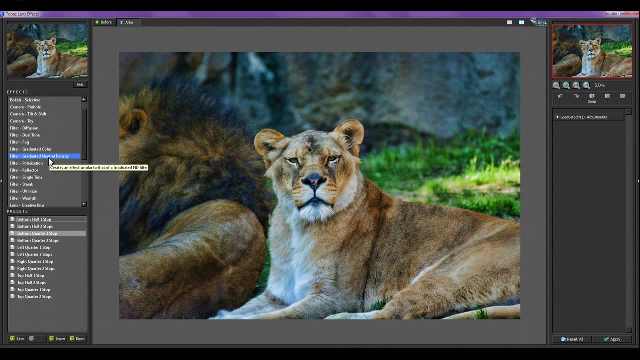 going to bring that back up. it's too bright for me. so, starting with the original photo layer, I'm going to go to lens effects and this, this little tool in lens effects I'm getting to show you, is really nice: the graduated neutral density filter. you can choose different places on the image which will darken. 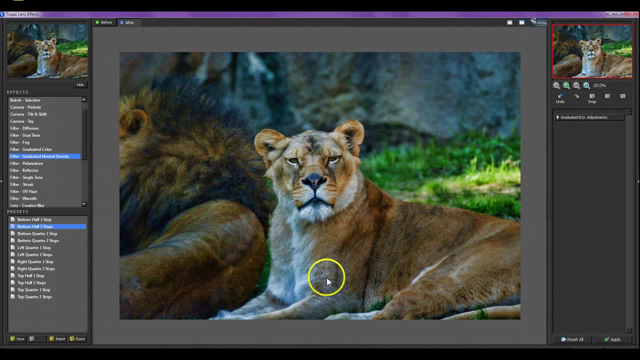 down that brightness. now that's darkening. bottom half, two stops. that's darkening quite a ways up. so I'm going to go to bottom quarter, which darkens right here. there's one stop. that's before, that's after. let's do two stops before, after. I'm liking the after on that one. so we're going to choose bottom. 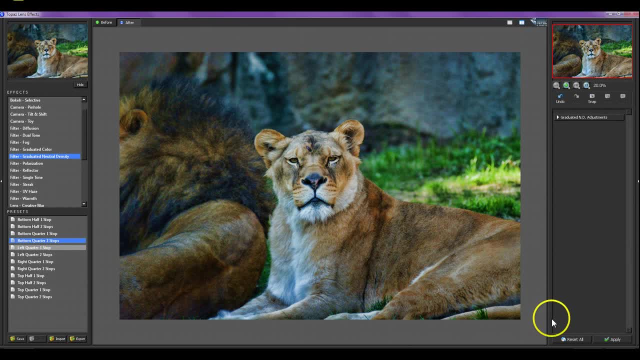 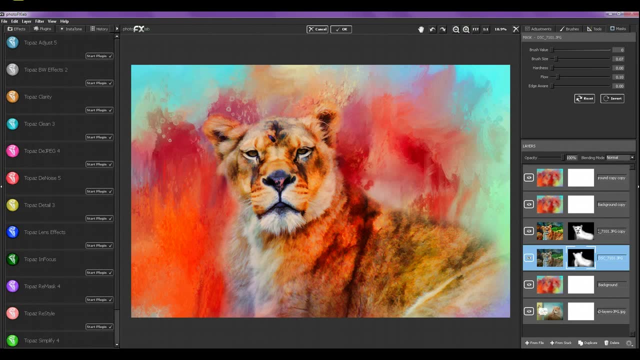 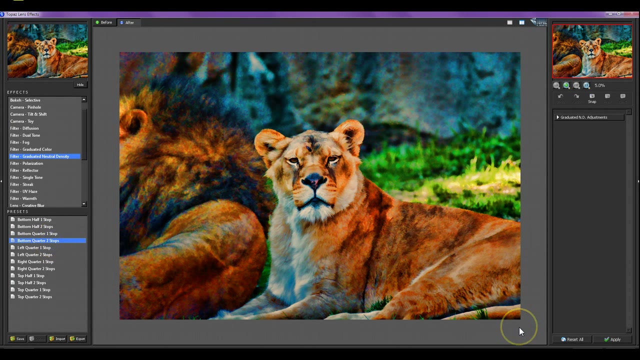 quarter two stops, which is going to darken this bottom portion by two stops on the original photo layer and we'll see if that makes any difference on this bottom area. well, that helped a little bit, but let's do the same thing on the painted layer. go to lens effects, bottom quarter, two stops. that's pretty dark. let's do one stop and. 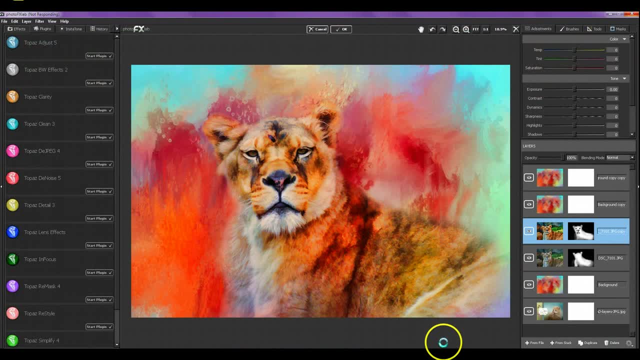 see if that's enough on that layer. that helped a little bit, but here's what I can do at this point. I'm going to merge them all, so I'm going to choose from stack and once this is all merged and the texture and the lioness are one, then I'm going to go back to 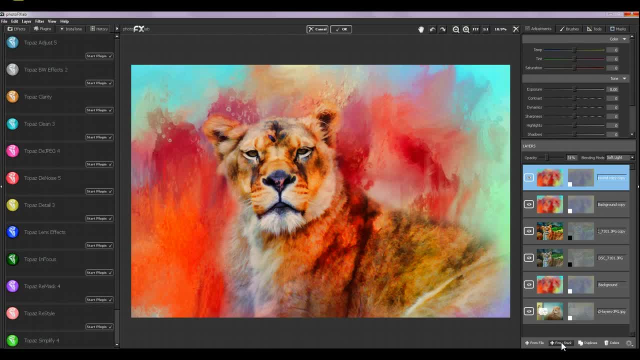 that lens effects and darken the the bottom portion here of the image. but it's gonna be of the merged image instead of the individual layers. rather than have to sit here and fool with those, I can go ahead and merge it. see what it's going to look like. 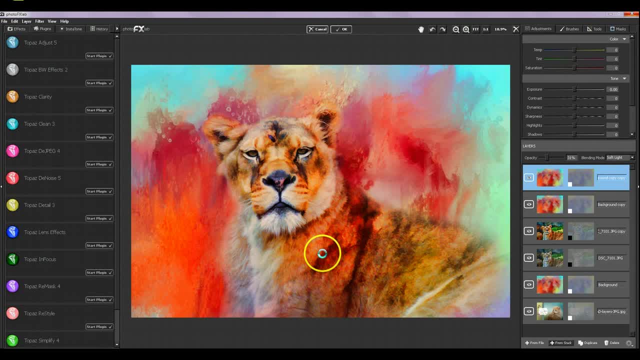 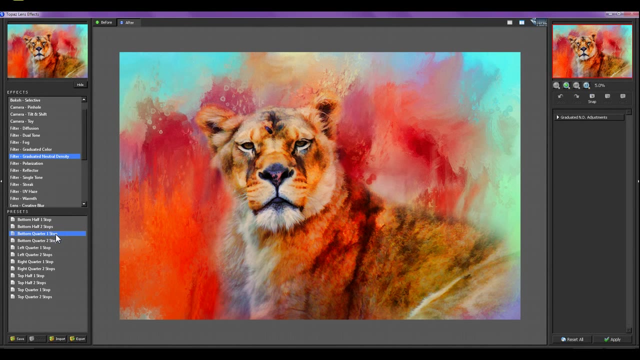 And one of these days it may get done. There we go. Okay, now we're going to go to lens effects, Now that everything's merged, and we're going to go to the bottom quarter. one stop, two stops. This is before, this is after. I think two stops takes away too much detail, So let's go. 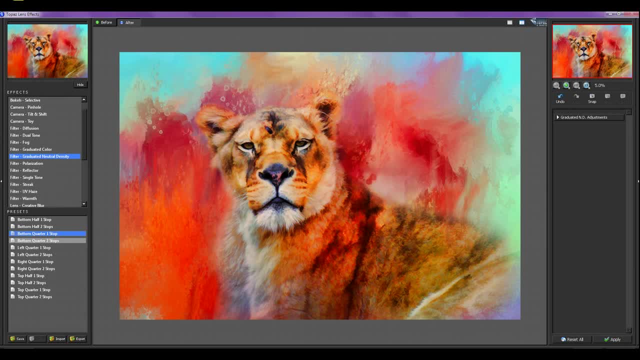 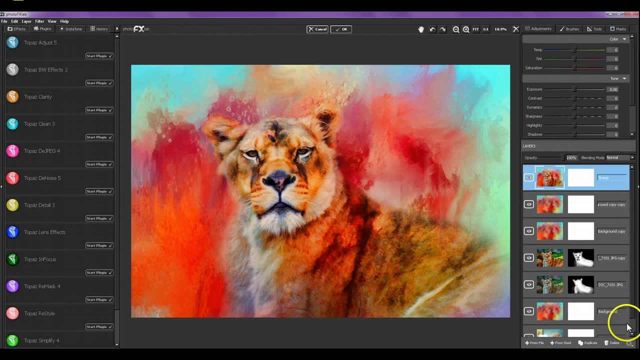 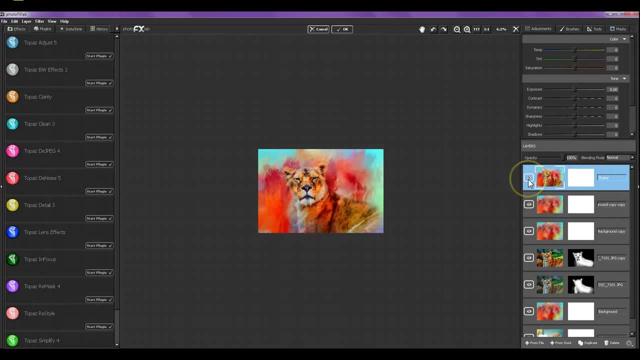 to one stop and try that Hit. okay, That darkened it a little bit more. So this is before, this is after. Let's zoom out to look at it from a distance. Alright, that's before, that's after. Now I could apply a vignette around the. 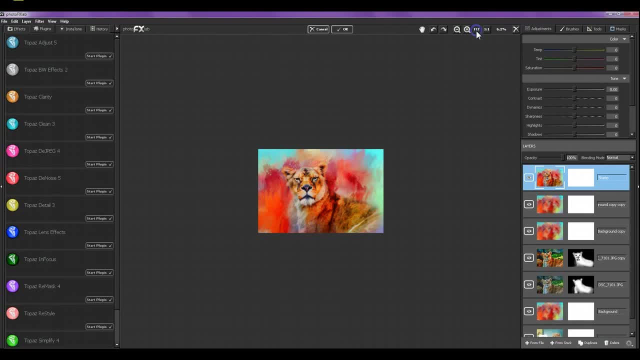 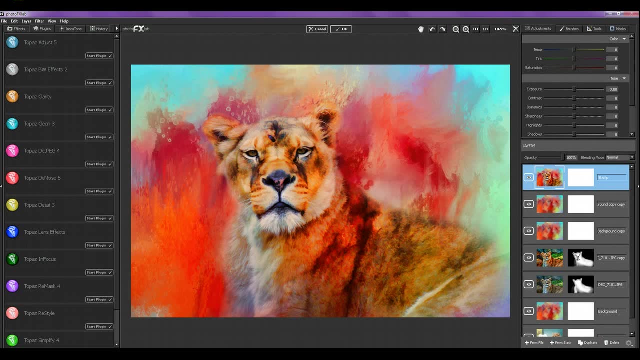 edges if I wanted to. but I don't want the other edges to be dark, just the bottom. But I could apply a vignette and then mask it away, except for just on the bottom. I'm going to try one more thing. I'm going to go back to the original texture. 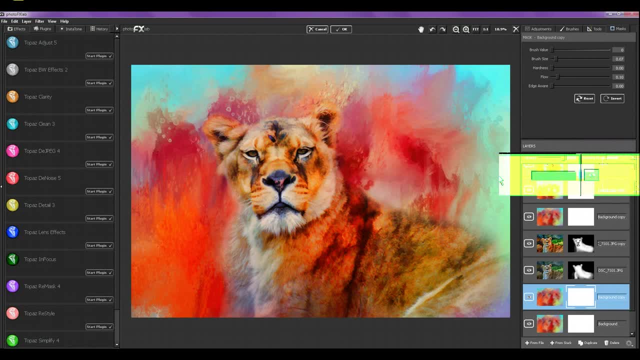 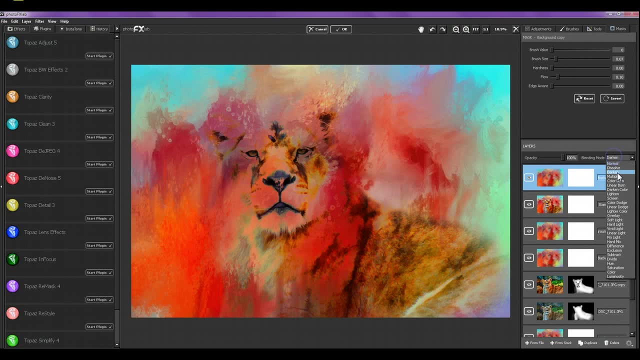 layer, duplicate it, bring it all the way up on top. If I can get it up there, There we go. Alright, now we're going to play with this. Oh, multiply, way too dark. Let's bring the opacity down. Bring it down to about. I'm just going to see if anything. 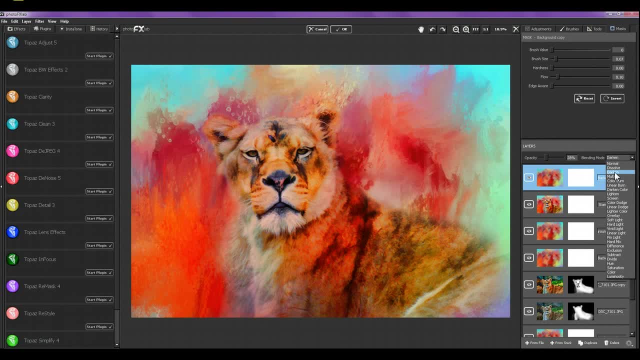 can be done here. There it is. I'll switch to Essex black and visual pliers Reverse. yes, and this is what I do. It's a bunch of playing. Funnest job in the world to sit here and play with these. I'm just going through the. 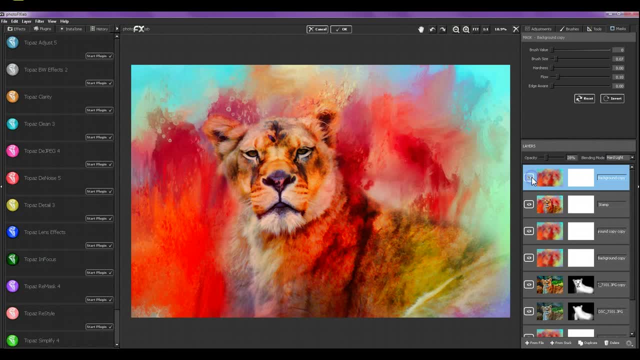 various layer modes to see if anything else might speak to me. Hard Light is kind of interesting. it adds a lot more texture to the lion. Yes, even at 30% it's darkening her too much. Alright, here's something I'm going to do, I think. 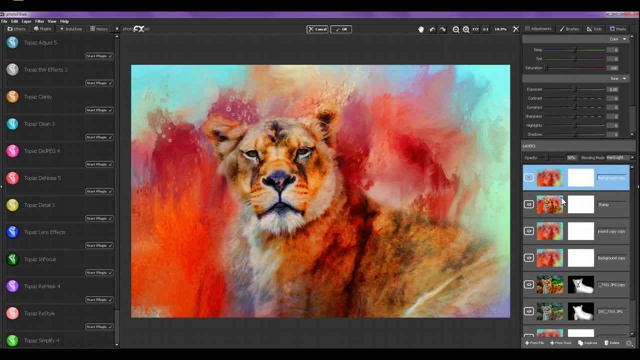 I chose the hard light. I put the texture back on top of my merge layer. I chose hard light at about 30%, which brought some of the texture back into the line, Gave her a little bit more interest. But when I had the saturation originally it was just too bright. 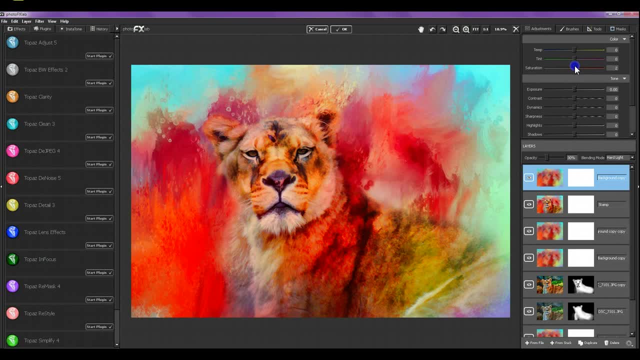 I mean, I like bright, but I don't want to go extremely overboard. So what I did is just brought the saturation of that hard light layer all the way down. Now, when I turn it off, you can see that that's what I originally had after merging. 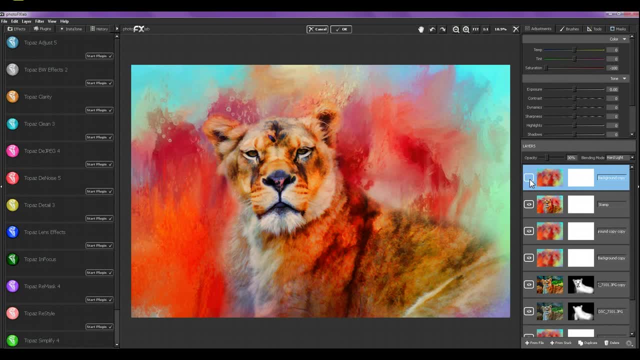 And now when I turn it on, it adds it kind of tones things down a little bit through here, But adds more interest through here. It shifts the light. basically is what it's doing. You watch her face right here. This is off and this is on. 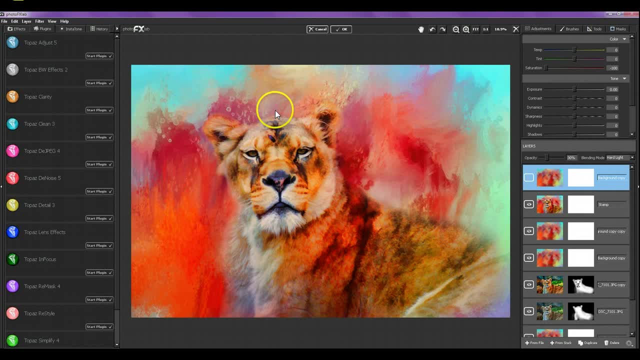 So it shifts the light and right now your focus is more on this side, where all the light is. But when you Put the hard light layer on, it brings the focus more to the center of her face And I'll just sit here and turn them off and on, off and on. 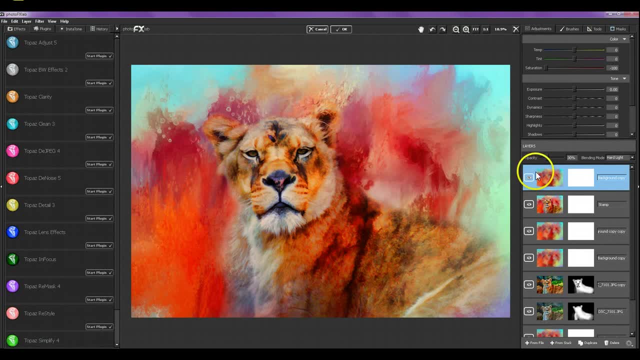 And it may be a little too dark now that I'm looking at it. One thing I could do is raise the exposure up of that layer, But nah, I don't like that. Let's see? No, because that makes her look kind of washed out. 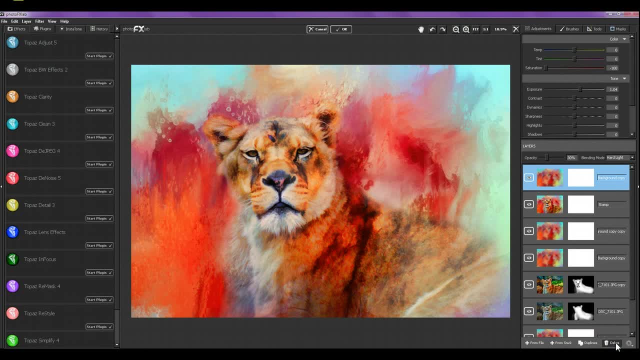 Nope, not going to do that, And that's part of what I do. Back and forth, back and forth. Put a layer on play with it, Adjust saturation, adjust exposure on the texture itself And see if I can come up with anything else that I like. 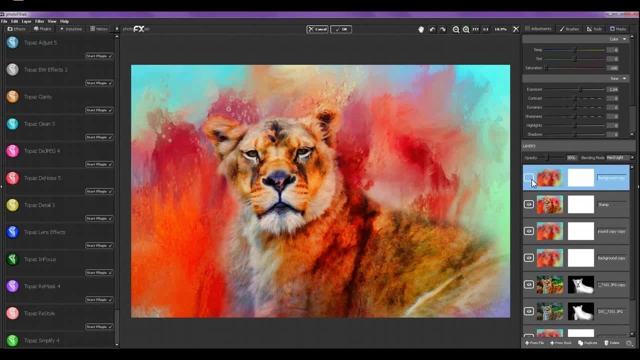 I don't particularly like this. now that I'm looking at it, I like the original better, that I had already merged, So I'm going to delete that layer off the top and stick with this. This is pretty heavy on the oranges and reds. 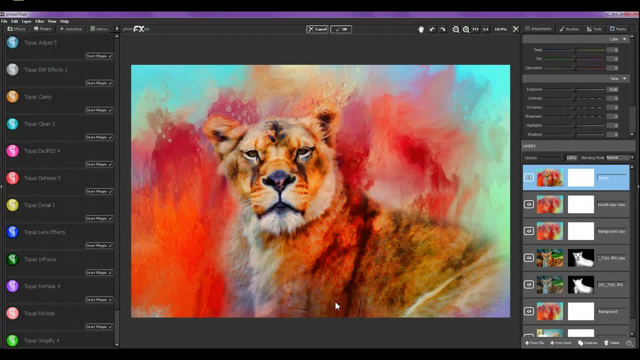 Which is kind of neat, Because that's that's out of the Summer Blast textures. most of them have had more of a goldish tone, except for the Summer Blast 5.. The one prior to this, which I am including in my blog post today. 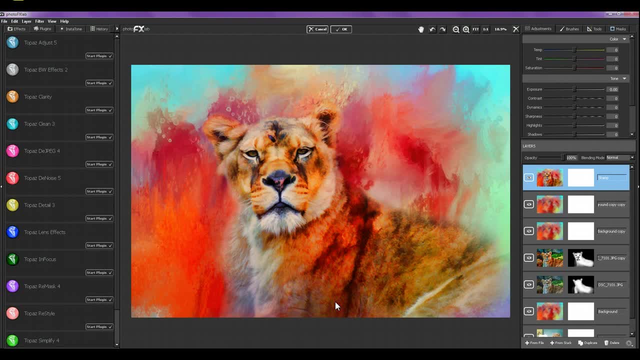 because I didn't make a blog post yesterday. it's a little darker. I'm liking this, though I'm just thinking if there's anything, Anything else I want to do to it, and I don't think there is at this point, I like it. 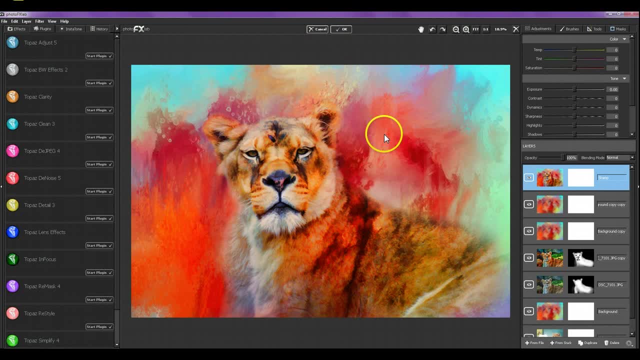 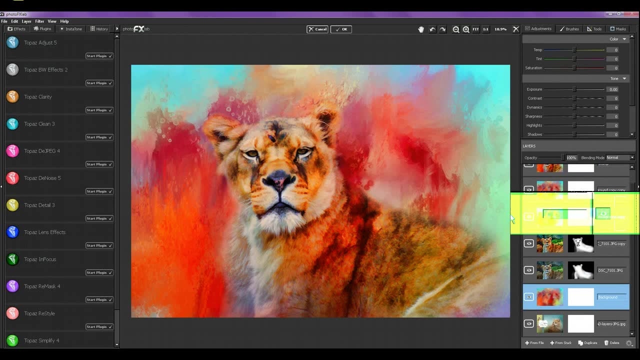 So at this point I would hit OK up here at the top and go back to my host program. But I wanted to show you something else. I'm going to duplicate the texture layer again and bring it. oh no, I'm going to duplicate it. 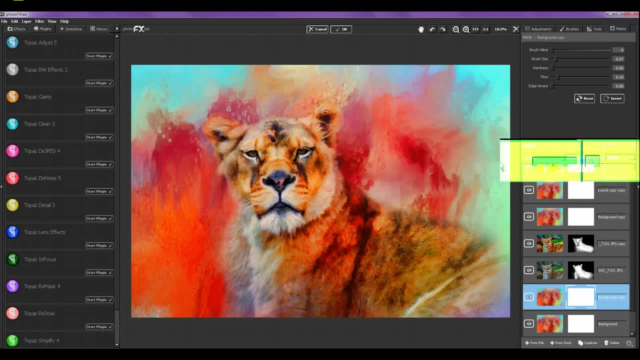 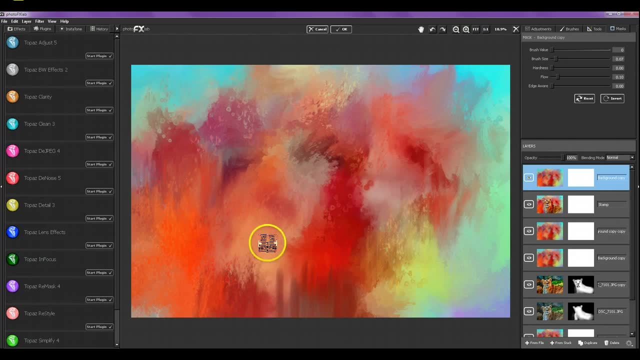 Not move it, duplicate it, Then move it. I'm going to put it up on top. So some of these textures here are, since they are so saturated and are full of color, if you like the texture, but that color is just a little bit too much for you. 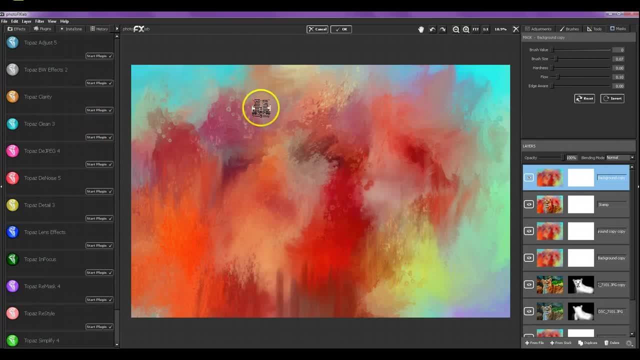 when you're first working with it. you have a couple things you can do, And I'm going to show you. this is going to teach you how to get a little bit more use out of the textures you buy, because you don't have to use them just like this, just like they are. 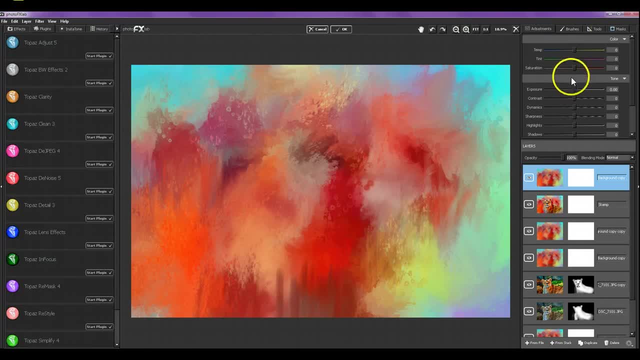 There's in your software. most softwares have a way to adjust saturation up or down, So if this was a little bit too saturated, you can adjust your saturation down And look at that. It's given it a lot more neutral tones, but yet the texture stays the same. 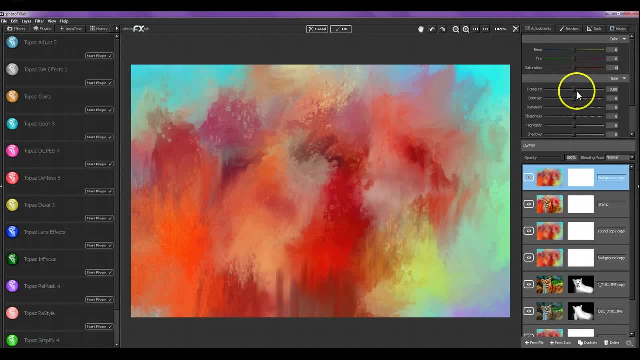 That's one way to handle adjusting it. Another thing you can do if you want to change something with the texture, actually making it become a whole new texture, is you could adjust exposure if you wanted to really darken it, Adjust it up if you really wanted to lighten it. 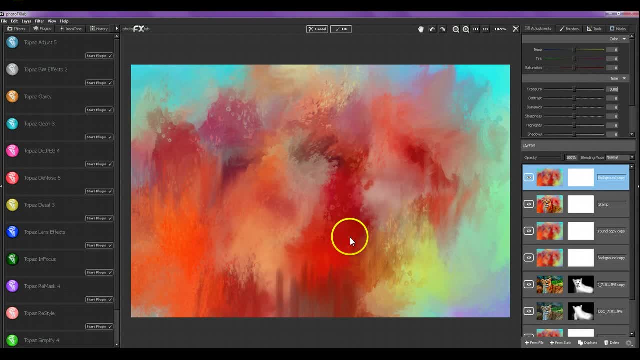 Now this is on just the texture by itself. If you're working with this and you're like now that's too much color for me, pull that saturation down and you'll still get the use of the texture. Or pull if you want a darker texture, if your subject is darker. 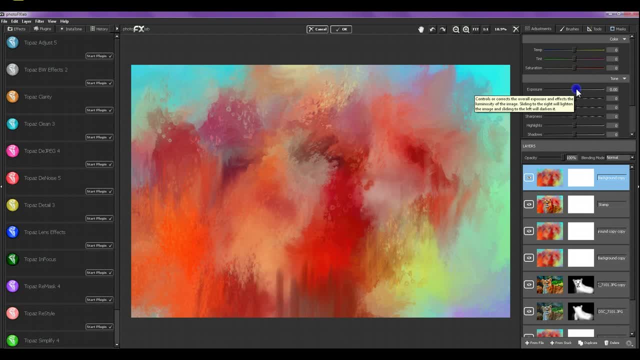 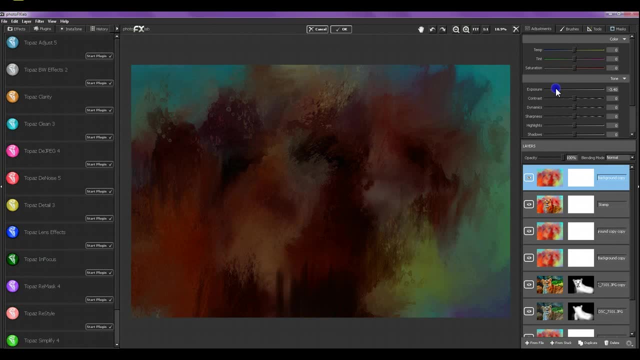 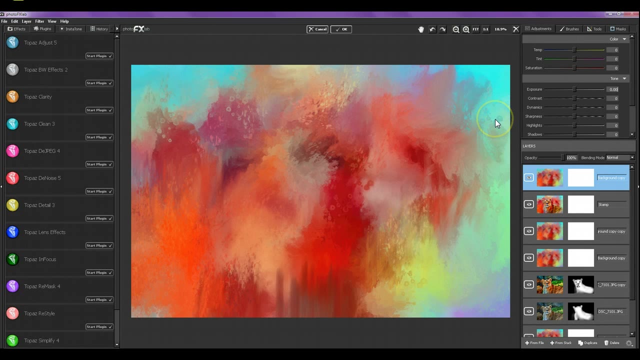 like a black animal or a darker scene, a night scene or something like that. pull the exposure down and darken it, Where you still get some effect from the texture but you're not losing the texture. So you can actually make adjustments to your textures and if you find one you like. 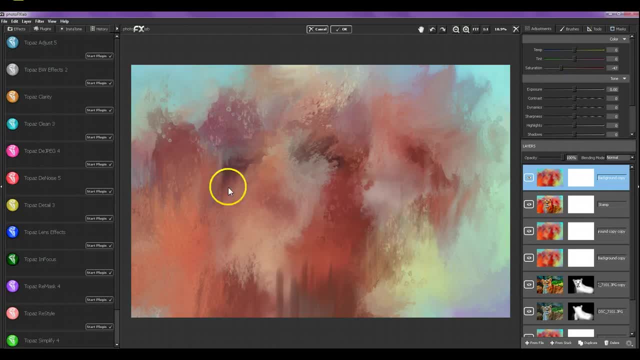 like if you pull the saturation down and you say, oh, I like those colors, they look more mauve and purple. now, If you like that, go ahead and save that as another file in addition to the original texture, and then you have a second texture you can work with. 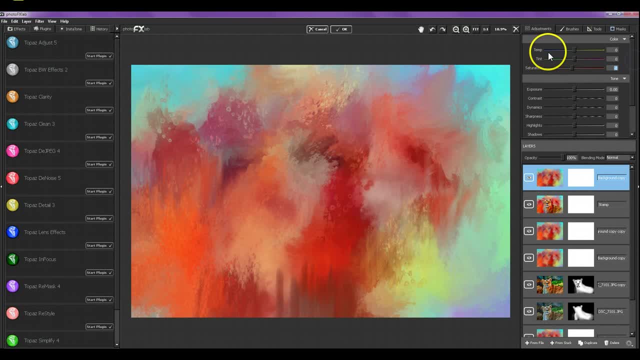 Just by making an adjustment in saturation, You can also adjust colors. You can adjust the tints and get real pinky and purple or fall colors. by adjusting tints You can adjust the temperature, make it warmer, make it cooler, and you can save all these variations as a totally separate texture. 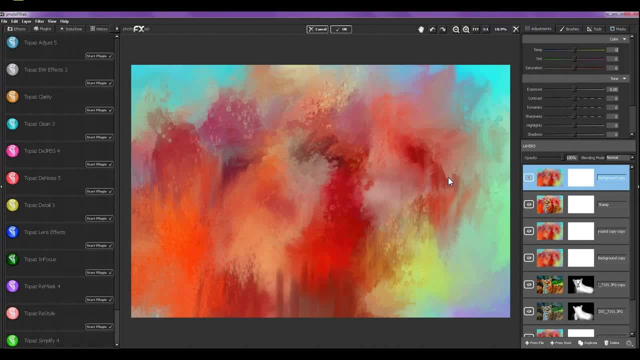 so that you can use it again without having to adjust it again. if you find that you like a a desaturated look more, You can desaturate this a little bit, save it and rename it as Summer Blast 6- Desaturated. 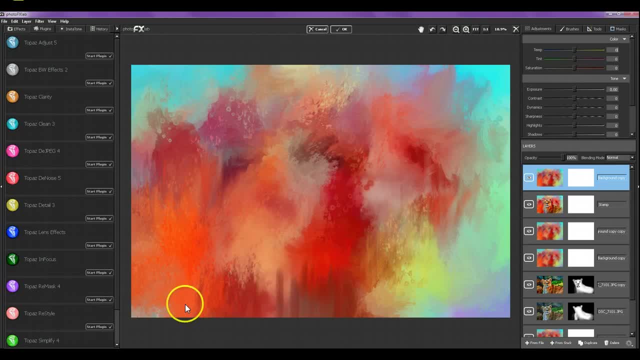 Now here's another thing that Topaz software has that I often will play with the textures. I'll like the texture, but it's not working right with the photo. I need to change color tones. I'll go to Topaz Restyle and this is amazing. 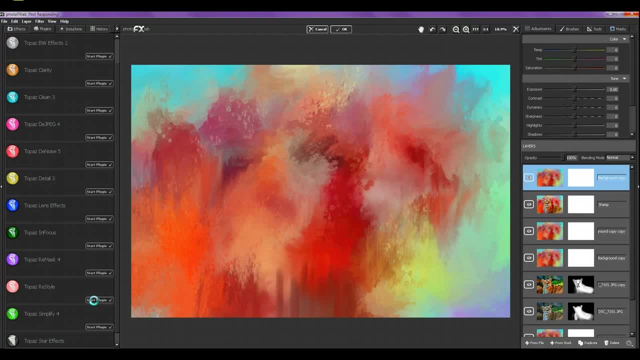 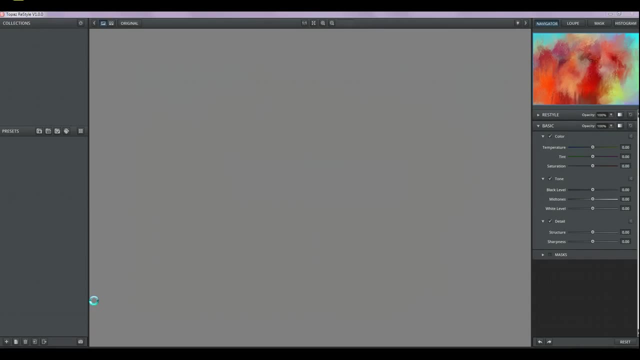 This Topaz Restyle, because this basically has a lot of color combinations. It's coded into the software that you can choose from that will allow you to change your whole tone of either a photo, a texture, a finished image. So let's say you you're doing an image for a client. 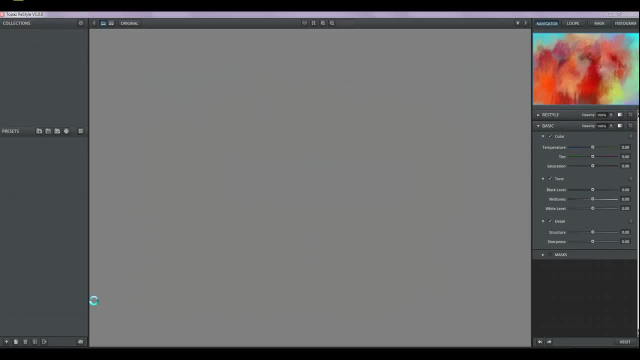 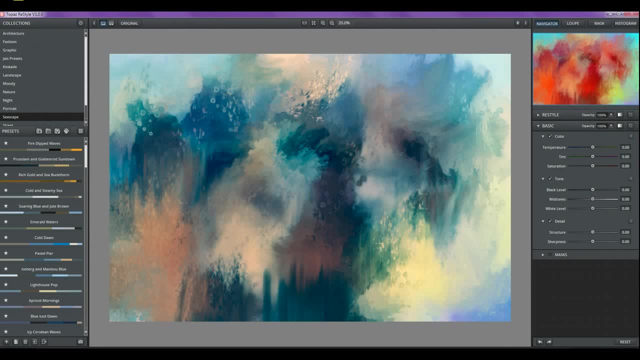 You do a real bright one and they're like: well, I like it, but it's a little too bright. I like more of the earthy tones. You can either pull down the saturation or you can go into something Like Topaz Restyle and you can. let's see, let's go to um landscape. 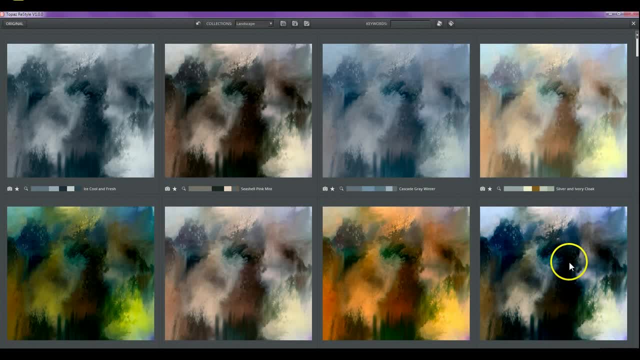 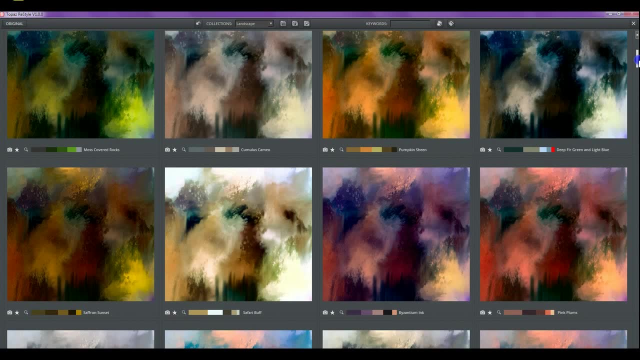 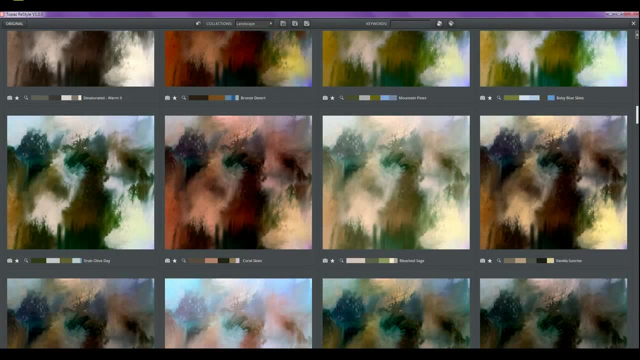 and let's choose. let's go through here. These are some of the landscape color modules. And let's say the client wanted something more earthy. You could um change the tone of your texture to be something More earthy, or your finished image, either one. 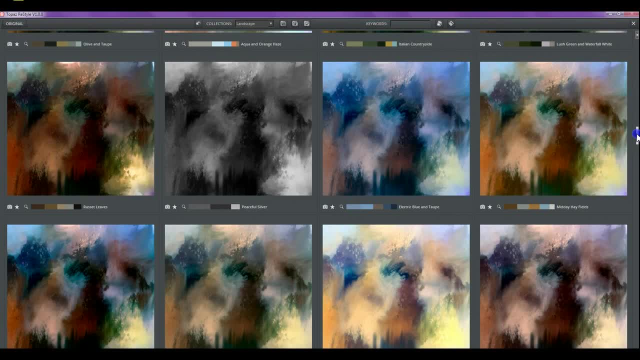 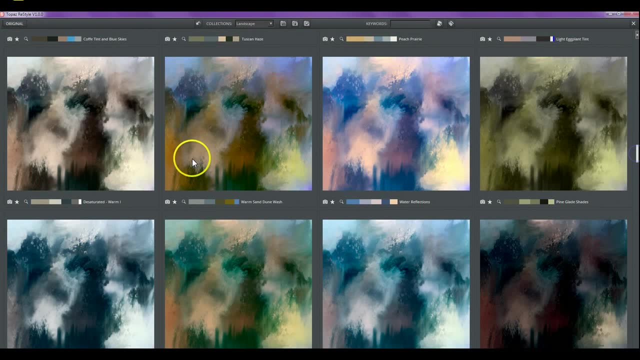 But look at all these combinations you can get by using Topaz Restyle with one texture. And so let's say you wanted something on the warm side, desaturated. you know that's a little bit too much, but look how much that changes. 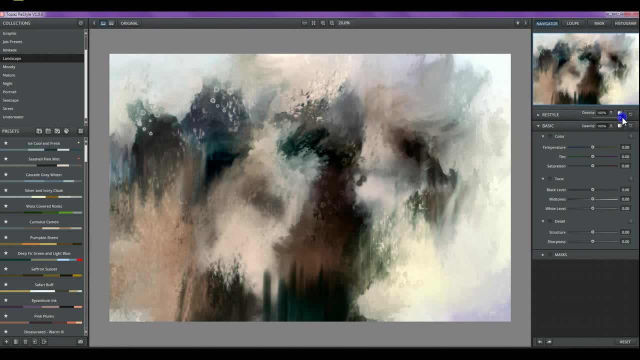 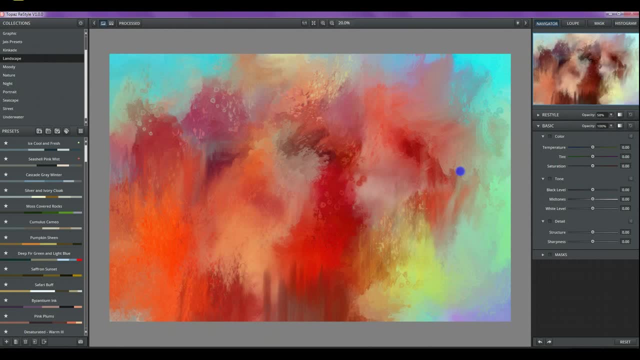 You can always adjust the opacity right here in Restyle too, Like, let's bring it down to this: Now you've gone from a really bright summer texture To a really interesting kind of autumn or winter, a mix of autumn and winter texture. 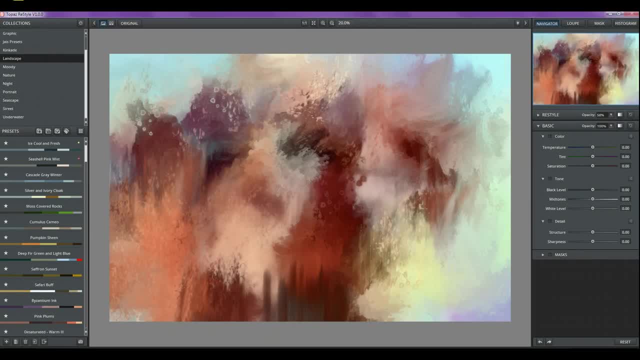 just by using Topaz Restyle And you could save this. if you wanted, You could click OK and you could save just this texture layer as another file. Name it, um, instead of Summer Blast 6,. name it Autumn Blast 1 or whatever you want to call it. 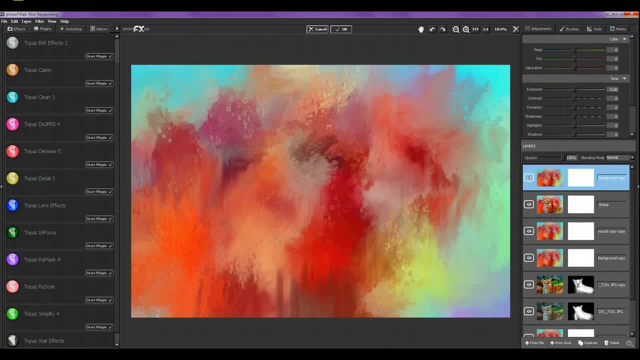 But it's. it's a way to textures that you can use With other images out of the same file. You can see it's. it's changed that. So at that point I could go to File and I could do Save As. 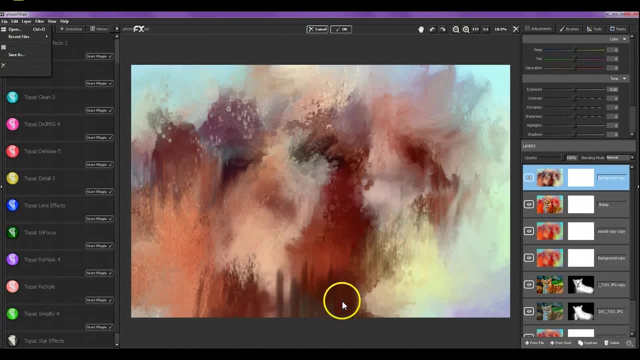 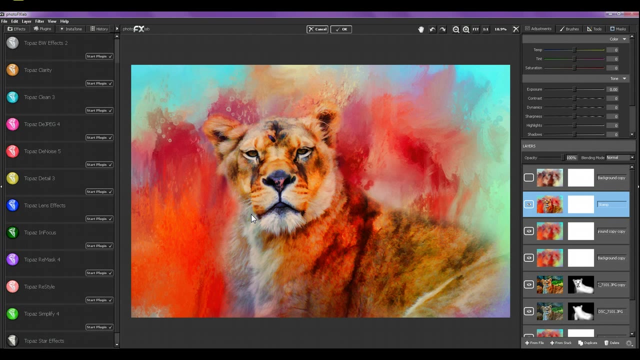 And I could save just this layer right here, um, and give it a totally different name. So then I could work with this with another picture, But let's just go show you, um, the finished image here. OK, here's the finished image that I came up with. 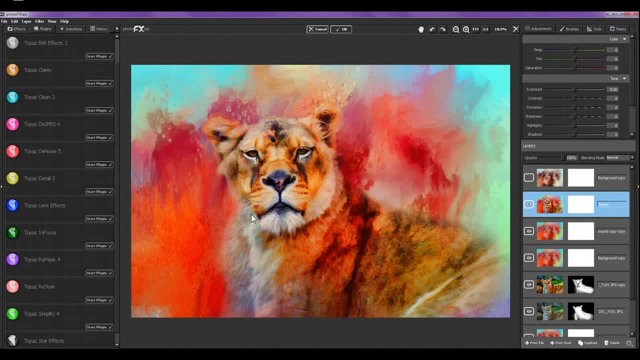 So let's say I was doing this for a client And the client says, oh, I really like this abstract look, but it's a little bit too bright on the oranges and the reds for my decor. I want something a little more earthy. 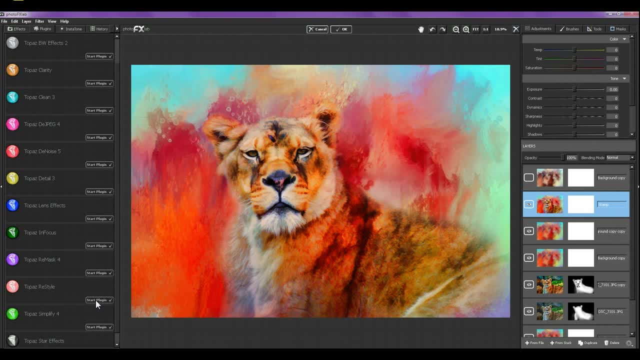 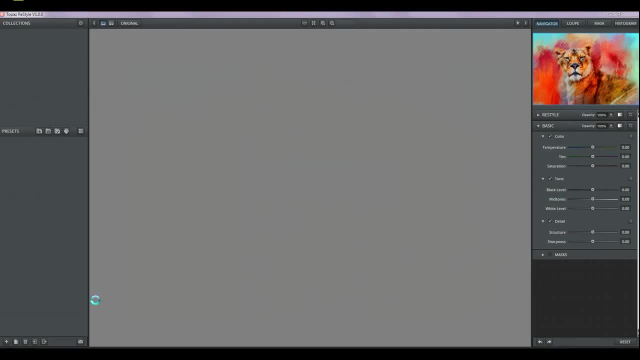 Take that merged image, go to Topaz Restyle, And you can do this in other softwares too. There's ways to adjust color hues, But let's let's go to Topaz Restyle And, um, if it'll ever open up, it should choose the last one I used. 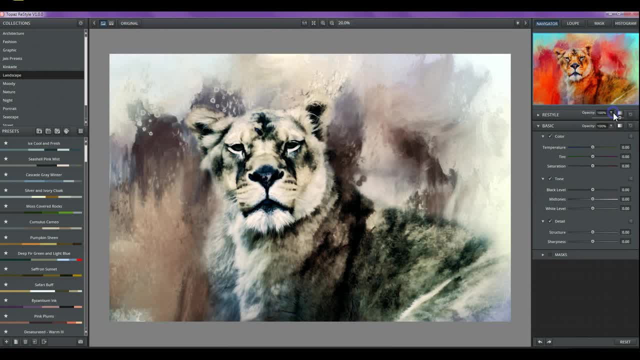 So that's the last one I used, but the opacity is at 100% And I reduced that example I just showed you down to about 50, 58% somewhere in there. So let's hit. OK, I should have duplicated this first. 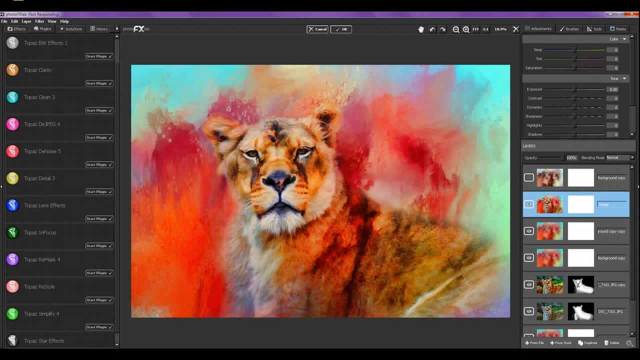 But I'll. I'll just undo it with a control Z because I want to keep my bright colored one. So let's say, client doesn't like the bright color one, It's a little bit too much. They want something a little more earthy. 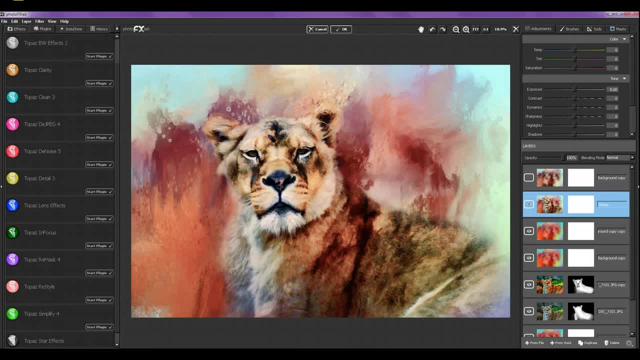 By using Topaz Restyle, you haven't had to redo the entire image. You can just adjust the colors of the same image, The texture- the texture is all still here. The abstract look is all still here, Just the color tones have changed by using Topaz Restyle. 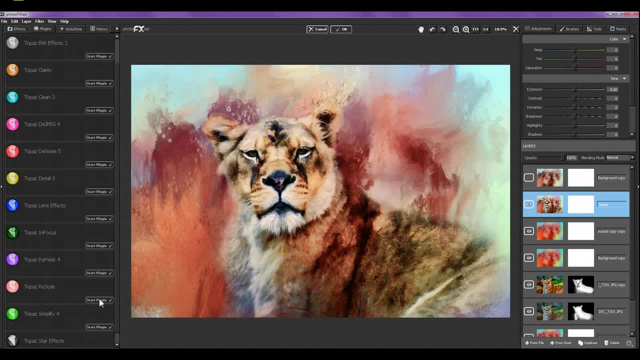 And you can use different comp. you can use it Different color combinations from, Restyle one on top of the other and adjust your layers. I mean your opacity of those different layers, But I like my bright one, so I'm going to keep it. 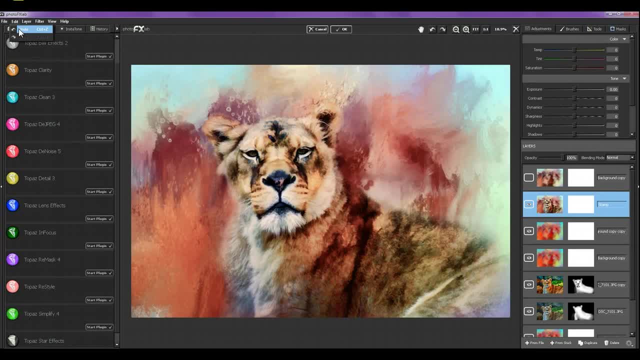 I just wanted to show you how you could get more use by adjusting color tones of the textures and still keep the texture itself. OK, we're going to undo this. go back to my bright image and I'm going to hit OK at this point. 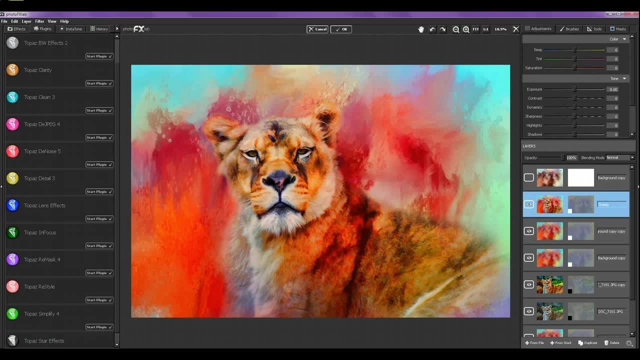 which is going to bring it back into, And I'm going to go back to my PaintShop Pro software. I know this video has gotten way too long. I really talk too much. I know some of you like it. I know some of you think man, does she ever shut up? 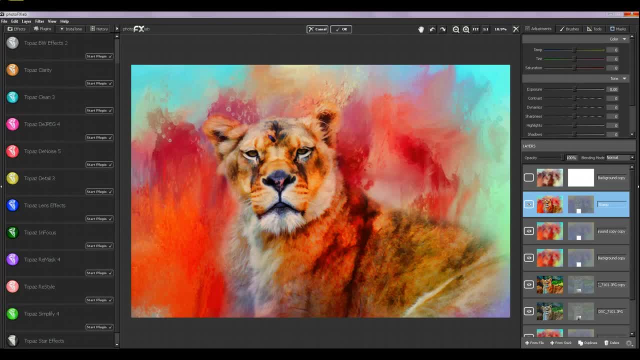 But when I'm talking about textures, no, I don't, Because I just love working with them. I love taking my photos and turning them into art, And this is a fun way to do it. There's so many things you can do. 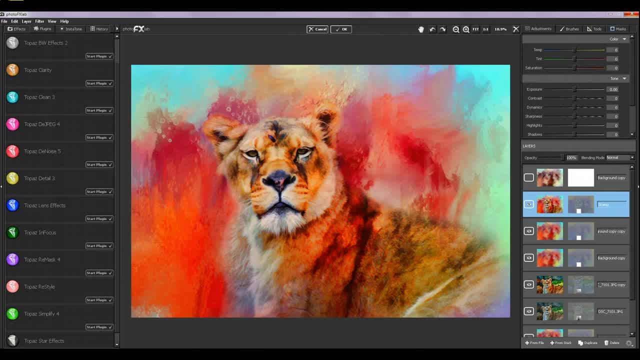 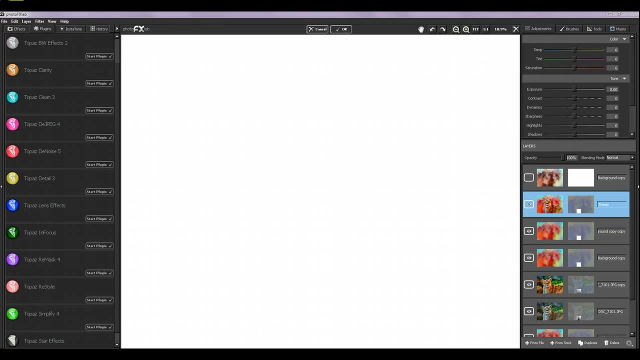 So many different combinations of things. you can do by using the textures and by blending them with the photos And, as this one proved, you can do another layer as a painterly layer and it will give your look that painterly look, but not over the top like some digital. 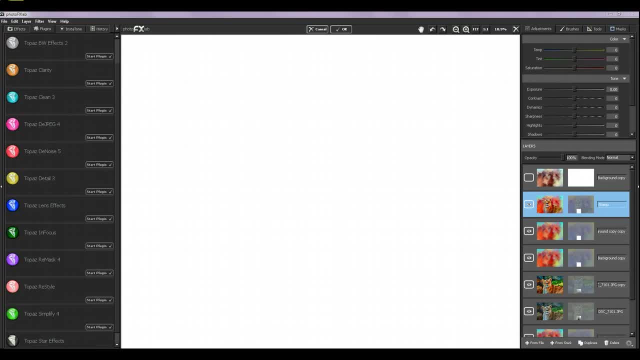 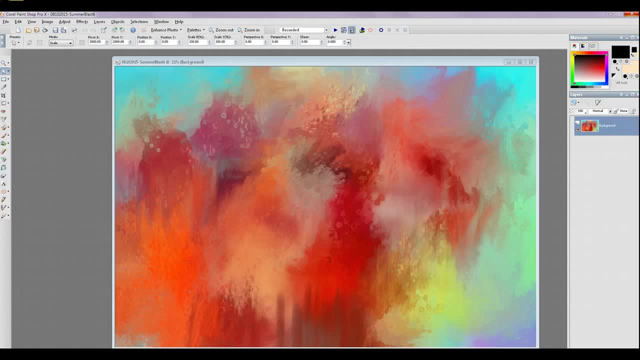 painting software will do when you tell it to auto process it. Sometimes it looks kind of over the top. By blending it with the original photo underneath it, you've toned down that that really computer painterized look and you've brought it. you've kind of done a mix. 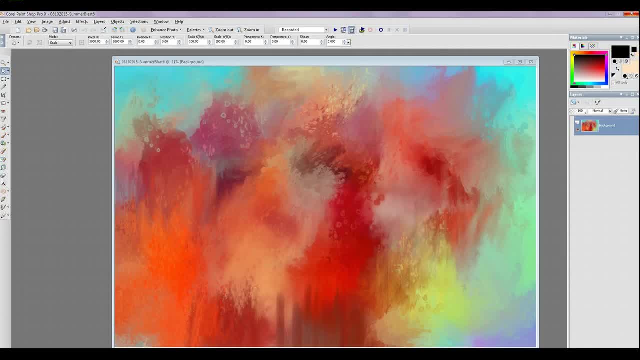 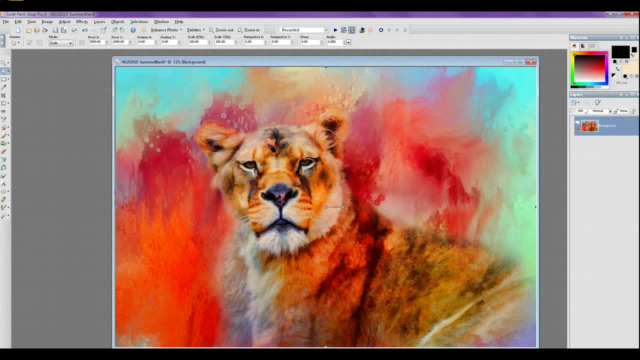 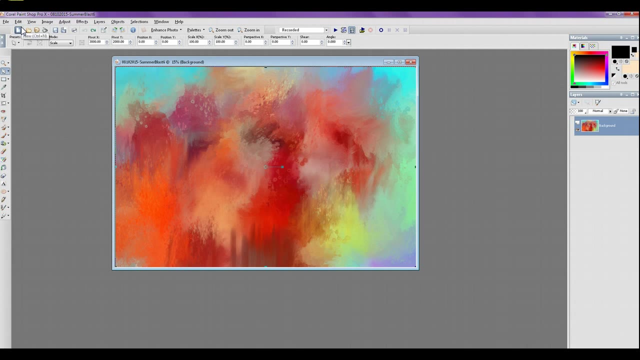 of that and the realistic, which softens it up a little and makes it look better, And this thing is taking forever to process. There we go. So there's my, there's my lion, And just to show you, that's the texture I started with. 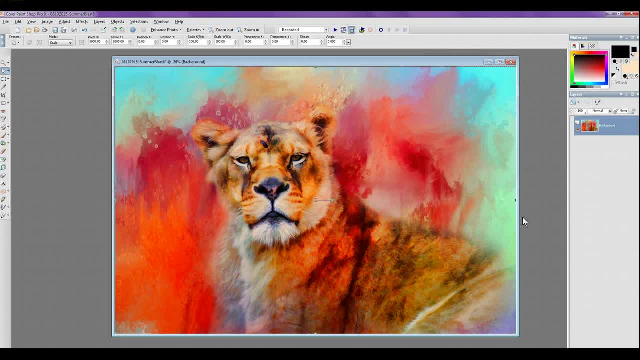 And there's my lion and I'm calling her done And I appreciate you watching. I hope this helps you feel a little bit better about working with these strong colors And that you will see that you can do a variety of type of images with these textures. 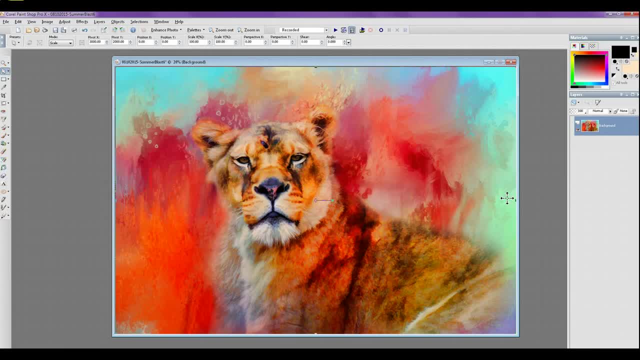 that are very strong colored, They work great. They work great on city scenes. not so sure about landscapes, but if you liked very vibrant landscape, they would work with that, especially in the overlay soft light or hard light modes. on top of a landscape, with just putting the texture on top of it. 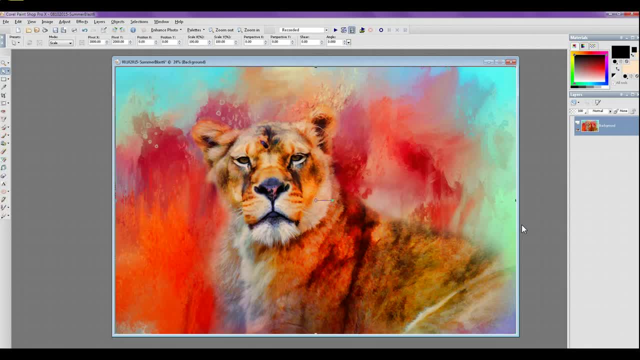 It can change the whole color tone of your landscape without doing any masking whatsoever. It can just throw some reds and oranges in that landscape. that may be kind of dull and you can brighten it up just by putting the texture on top as a certain layer mode. 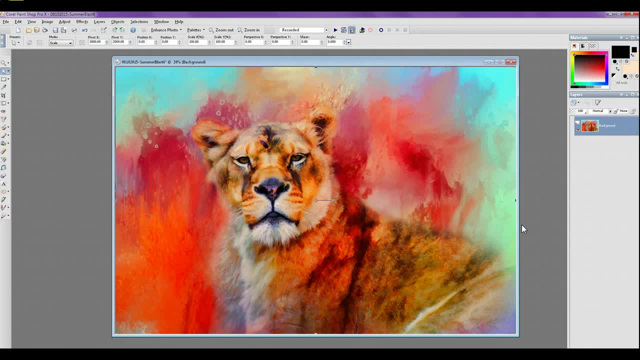 And then you can, of course, use it like I have here and blend it with a variety of subjects, And this whole color expressions line of work that I'm doing is I plan on doing a whole lot of subjects using this method and using these very bright, saturated 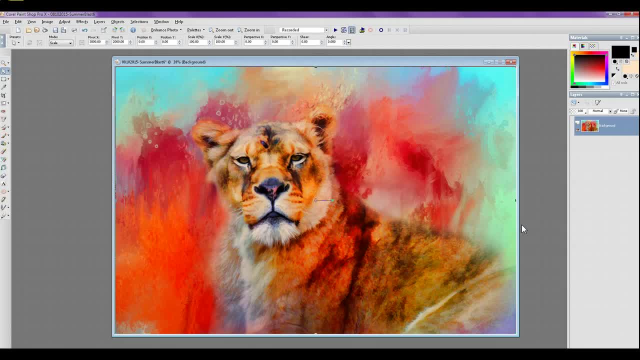 colors. Um, the very bright, saturated colors are very commercially appealing- I guess is the word right now- and I've been wanting to do these for a while but I've kind of been scared that like that was too much color. But people really like them and they look really good on lots of fun products like pillows and 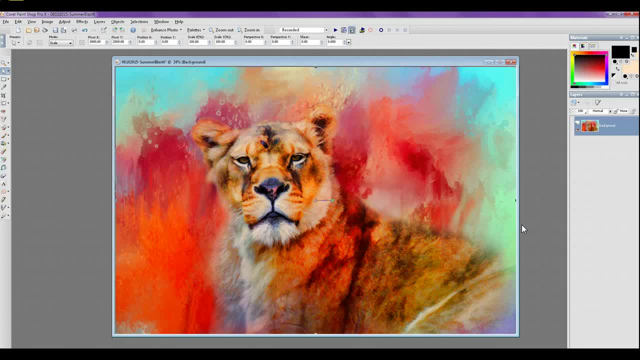 rugs and blankets and you know the art prints, of course, but there's so many other products that- But this particular style image just really looks fun and powerful on those other products- Coffee mugs, child trivets, things like that- And they just really make the products come to life when you put these type of images on those products and they're very commercially appealing. 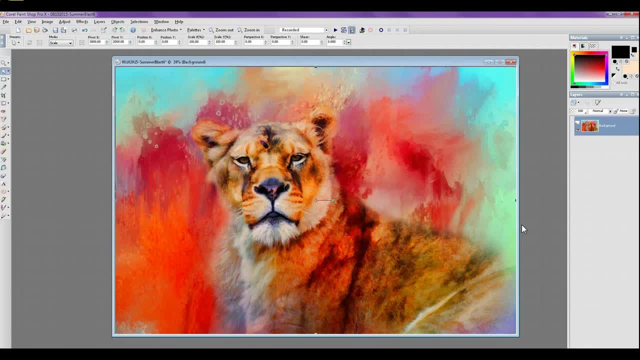 So that's why I wanted to do them, But I plan on doing lots of wildlife: dog breeds, songbirds, the birds of prey. of course That's being included in the wildlife. I'm going to do some other subjects too, in the same manner. For instance, some food subjects like cupcakes and fruits, And I have a whole list here somewhere of different ones: Flowers, seashells. 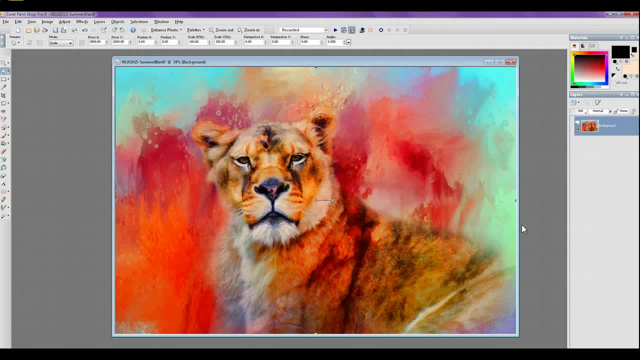 Just things like that that might blend well with these type of textures, Because I have photos of all of these things And I'm just looking on a way so they get a little bit more exciting look and they become more commercially appealing, And these bright colors really do that.